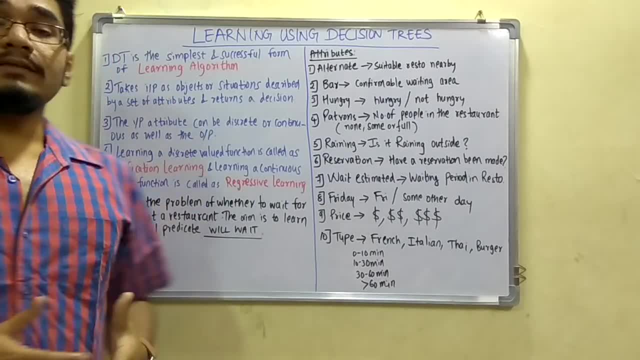 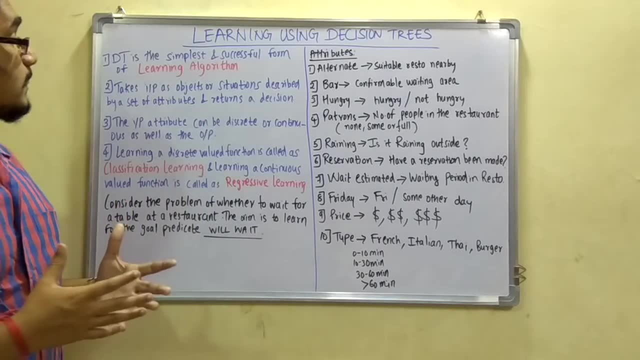 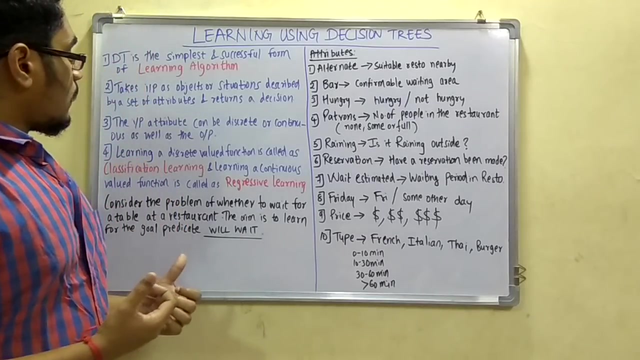 trees, that is the DT in short form, is the simplest and the most successful form of machine learning algorithm. basically, Now, this decision tree takes input as situations or objects, as described by any of these attributes, and returns a particular decision. Now the input attribute can be discrete or as well as continuous. 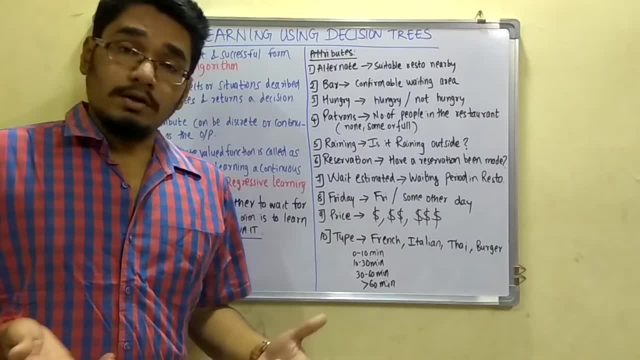 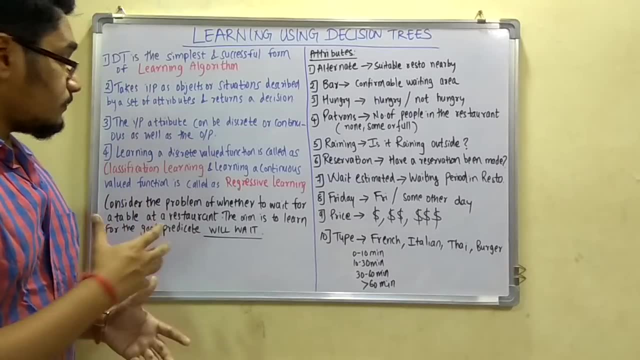 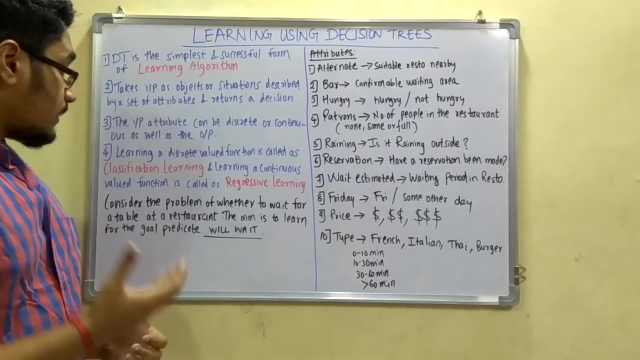 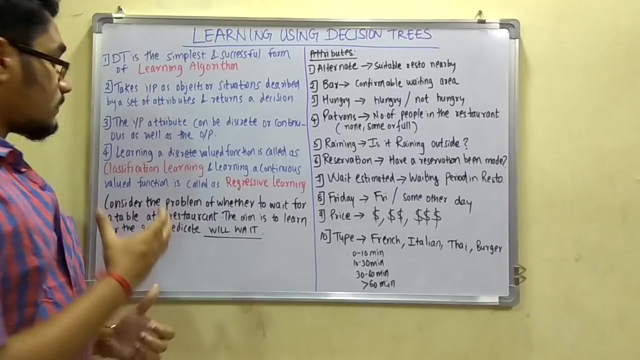 As well as the output, can also be discrete or continuous. Now this learning using the decision tree by using the discrete valued functions are classified as the classification learning, and learning using the continuous valued function is classified as the regressive learning. Why the discrete valued function is classified as classification learning? 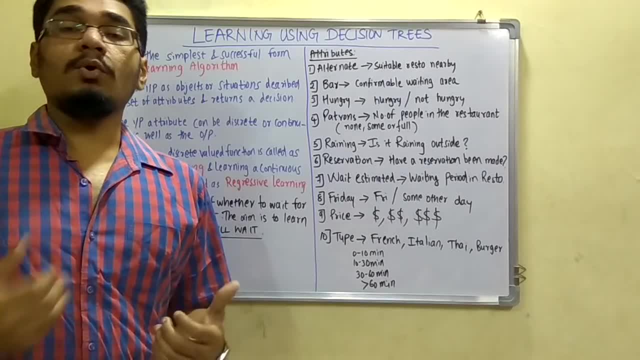 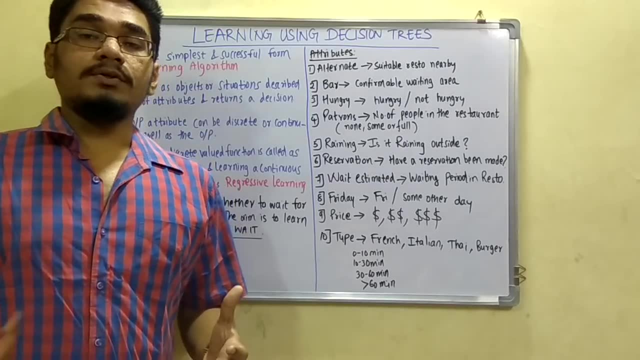 Basically it divides the decision tree into two parts. The first part is the learning that gets it into certain domains. So by these domains we can actually come to know that in which category this learning is fall into. so that is called as the classification. 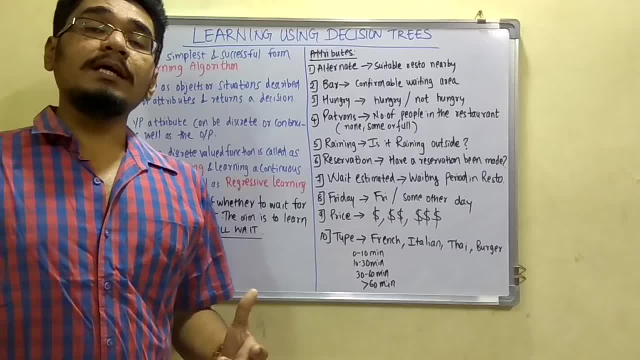 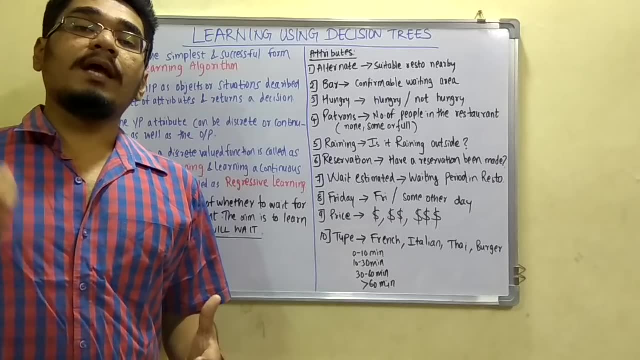 learning, and the learning is in continuous valued function. It will be a graph, moreover, and that will be regressive. learning means more and more. When you refine it, you can add new ideas or new decisions can be more clearly taken, So it comes under the regressive. 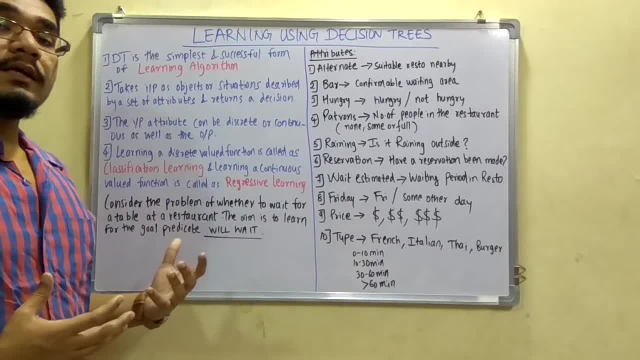 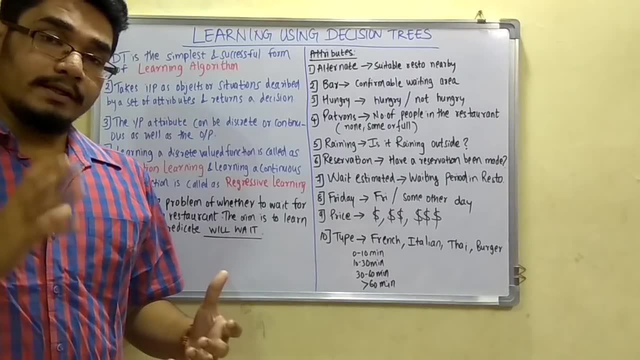 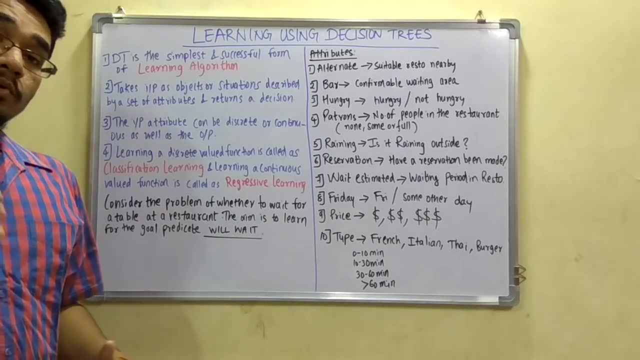 regressive learning. Now, all this under comes under the example of the decision trees. Now there is a problem of restaurant in decision trees which we are going to solve. So consider this problem of whether to wait for a table at a restaurant. Now our aim is to learn for the goal. 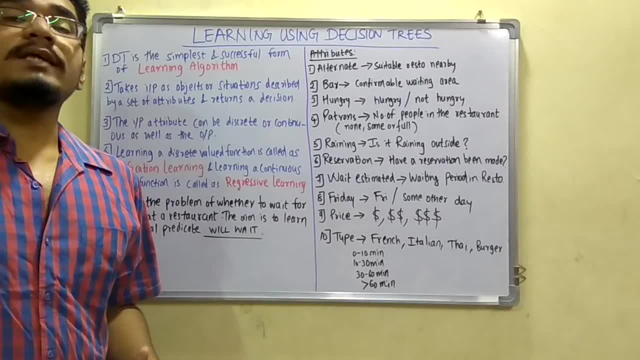 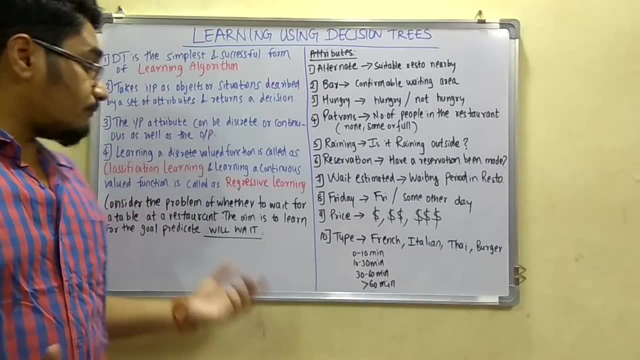 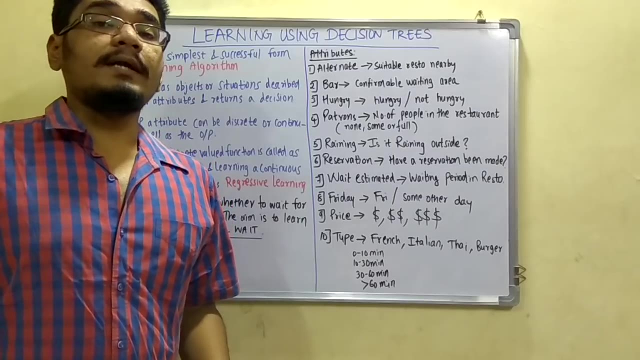 predicate, that is, the machine will have to decide that when it reaches the restaurant and it searches for a table, it has to decide whether it will have to wait or not. So to consider this decision tree, we consider certain attributes for designing them. So there are basically 10 types of attributes, as 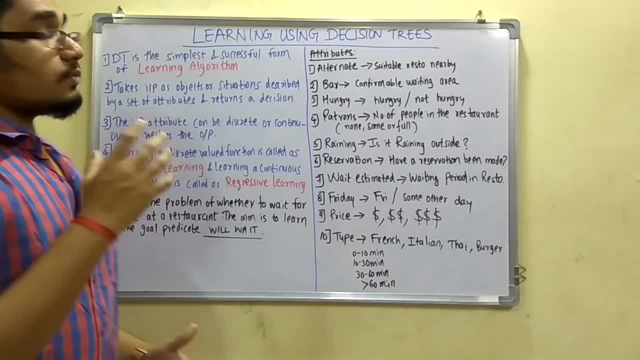 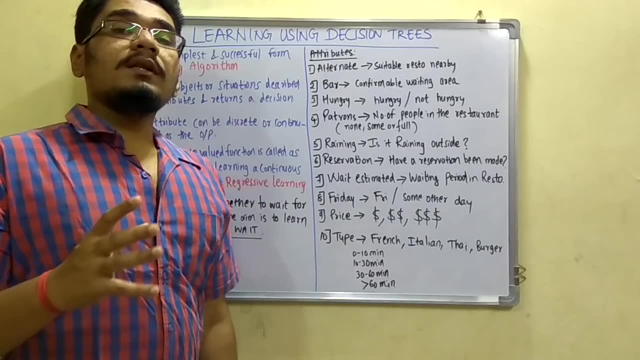 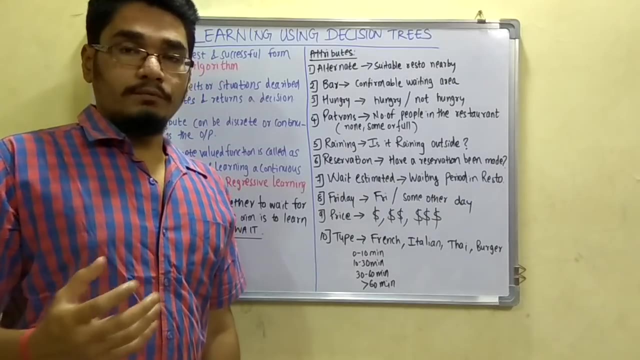 listed here. Let's see one by one. what are those So, first of all, the first attribute is the alternate. Alternate means if there is a suitable restaurant nearby, not very much long distance, but it should be in a few kilometers, within a few kilometers, So that comes under the alternate. 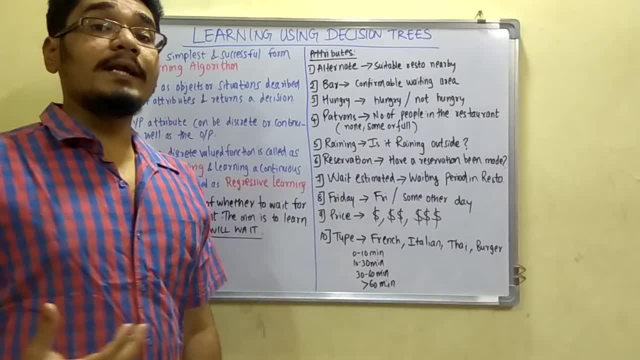 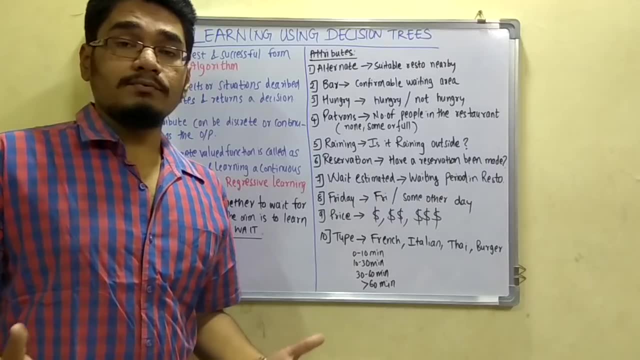 attribute Next is the bar attribute. Bar attribute states that whether that restaurant has a confirmable waiting area means if the restaurant is full, then whether the patrons can wait for a few minutes or for a few hours. So that is the first attribute. Next is the bar attribute- Bar. 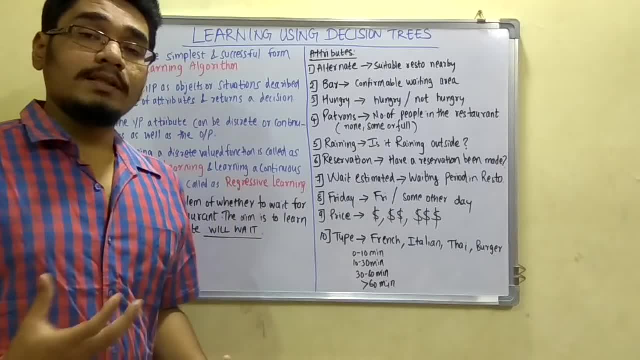 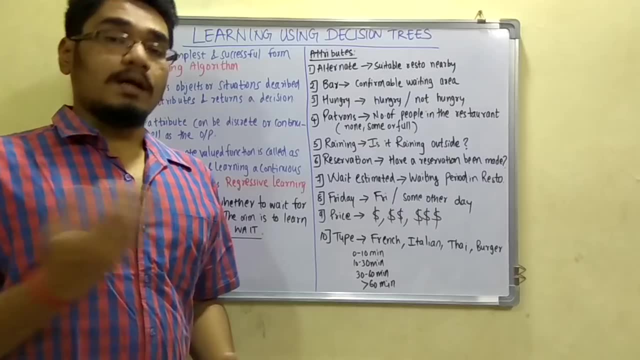 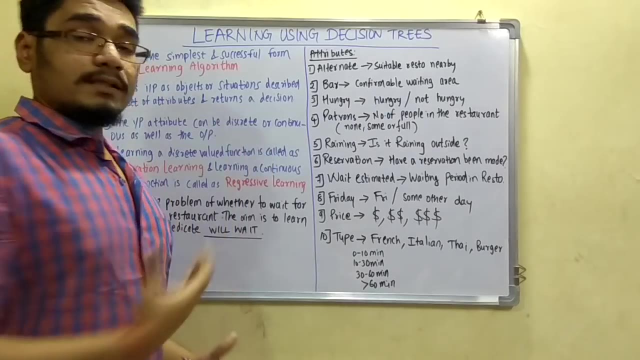 attribute states that whether the patrons can wait for a few seconds. So that's what the bar. And next is the hungry. whether the patrons or the persons are hungry or not, Whether they want to leave or whether they want to still wait, It comes under hungry. Next is patrons. Patrons are those 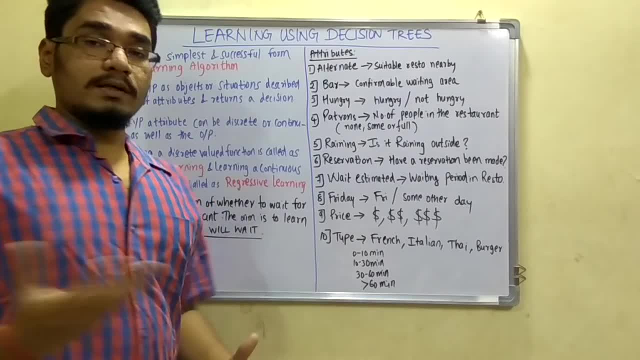 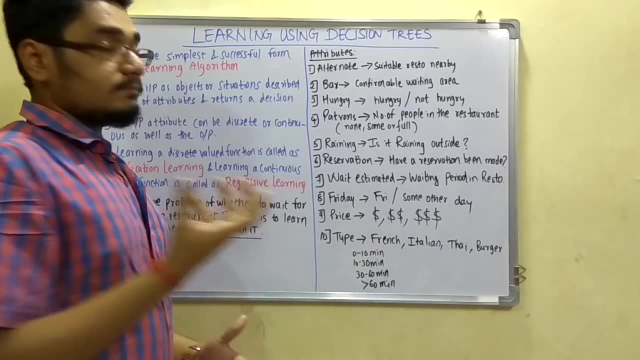 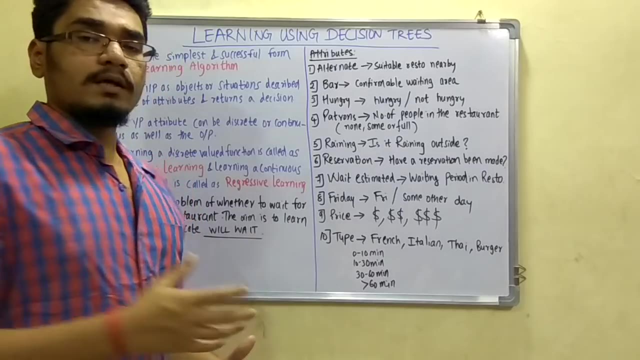 the number of peoples who are visiting the restaurants, who are sitting or who are waiting outside the restaurant in a bar. So it values the number of people who are sitting or who are in the restaurant, whether it's empty. Also, the bonus attribute Values Can be none same or full. 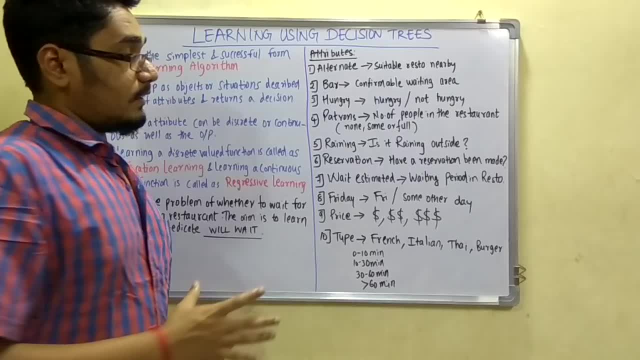 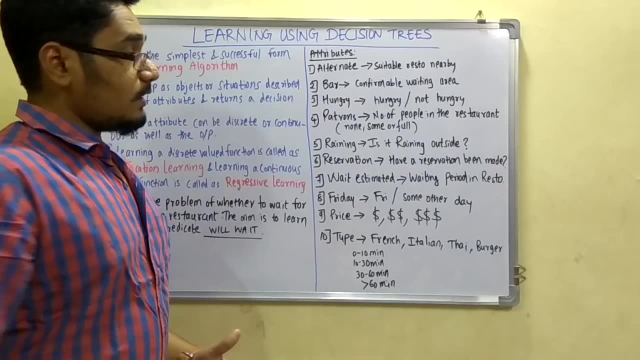 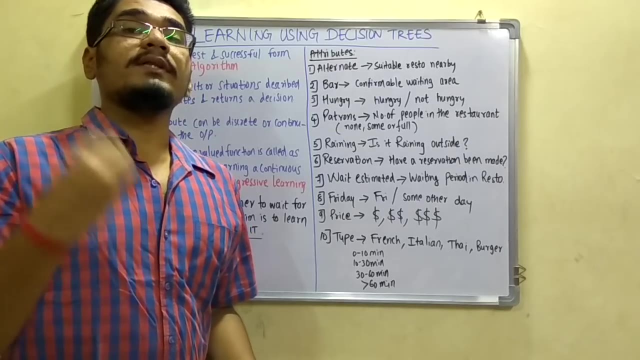 means no persons are there, or are a few persons, or the restaurant is houseful. Next is rainy. Now, if it is raining or not raining, whether it is a winter or a fall. Next is reservation. have somebody reserved a seat for a restaurant? means Already someone has been booked, or whether they want toフَنا, coupled to the boarding and restaurant must perform an. 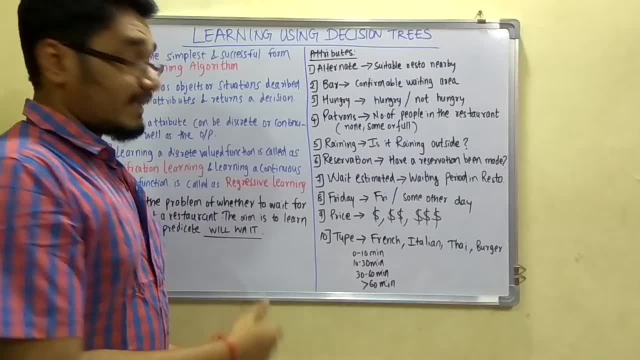 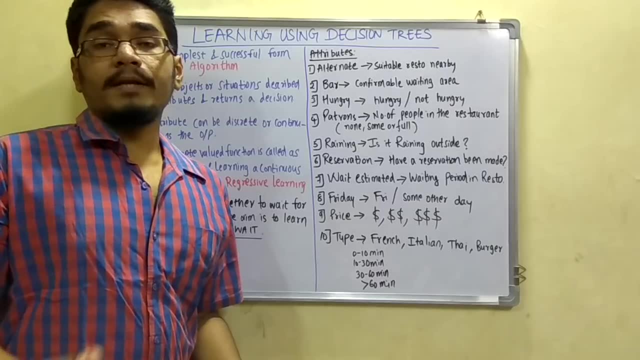 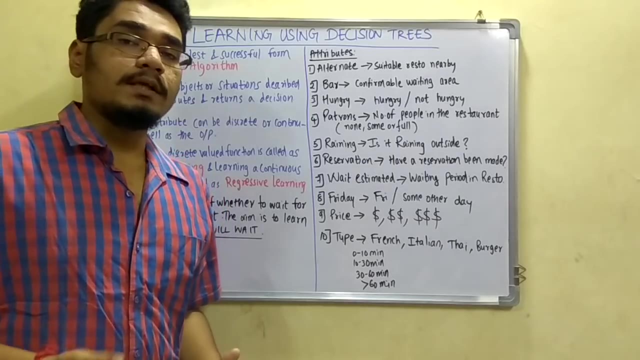 have the table, so that comes into reservation. next is the weight estimated now. waiting period in the restaurant means, when a patron or certain patrons arrive, whether they have to wait for a particular period of time or whether they can go immediately into the restaurant for having the food, so that 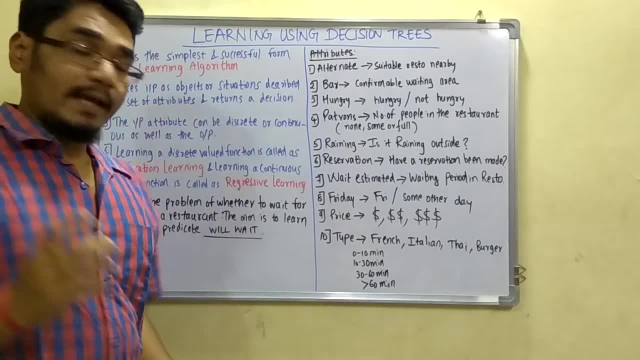 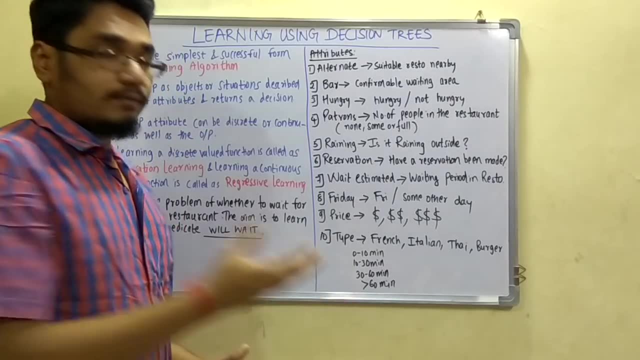 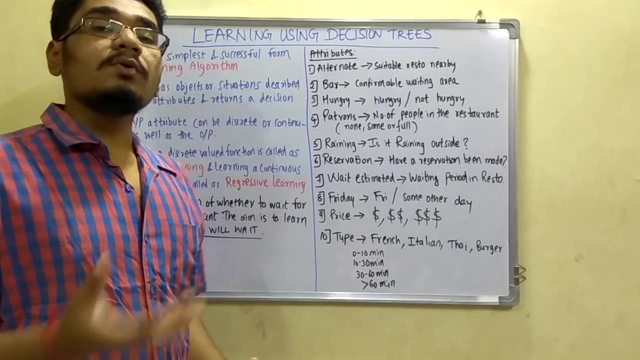 is estimated by a wait time. now this wait time is measured in four categories, or it is categorized into four. that is 0 to 10 minutes, means it is reasonable. 10 to 30 minutes, it is somewhat 30 to 60 minutes. it's almost one hour. no one will. 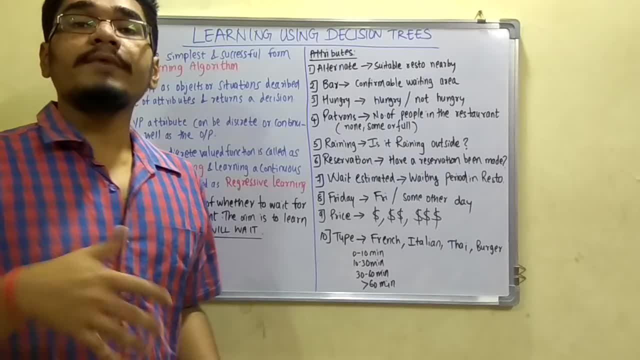 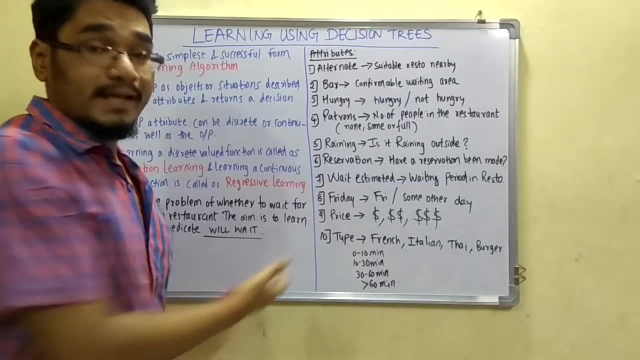 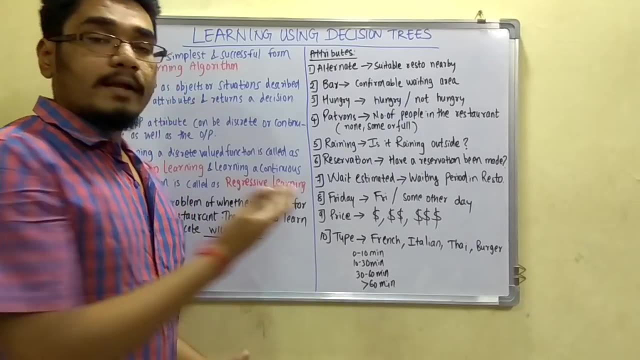 wait for that much time and more than 60 minutes. no one ever will wait for more than that much minute. next is we consider some additional attributes, like the days, whether it is a Friday or some other days, a public holiday or some other day. next is the. 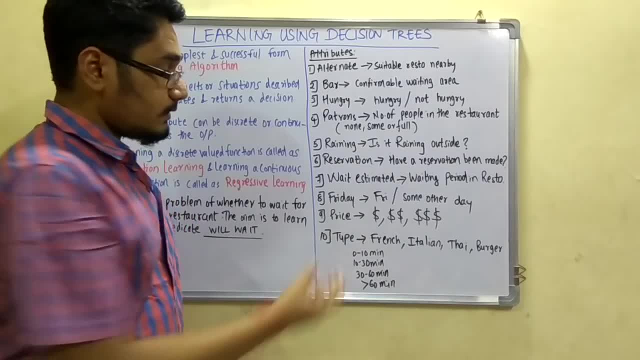 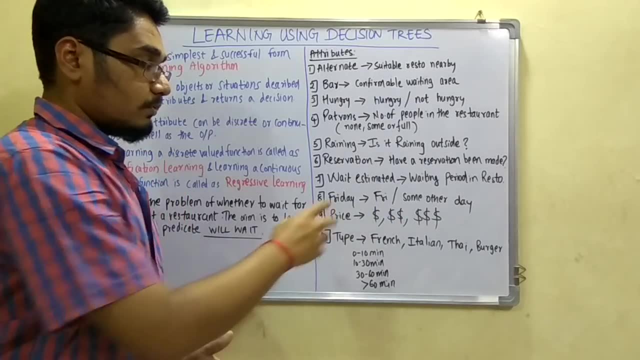 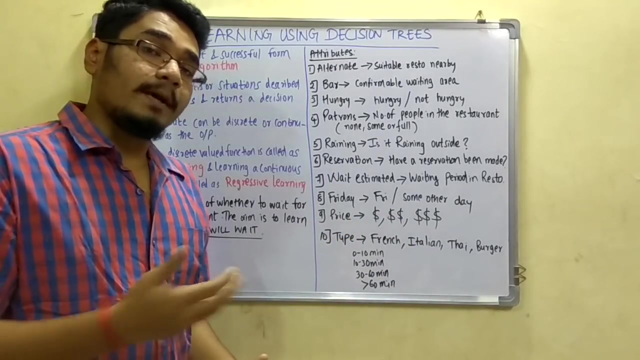 price, whether the price is reasonable, whether it is of some dollars, $2, $3. the dollars indicate the hundreds units or the 10, so that's why it is single dollar, double dollar and triple dollar. next is the type, means the type of food which the patterns are going to have, so it can be the French dish or the Italian. 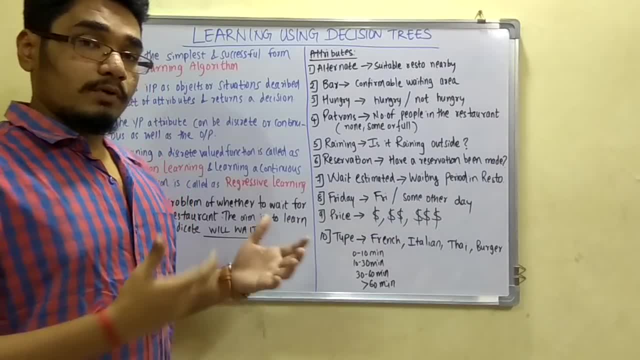 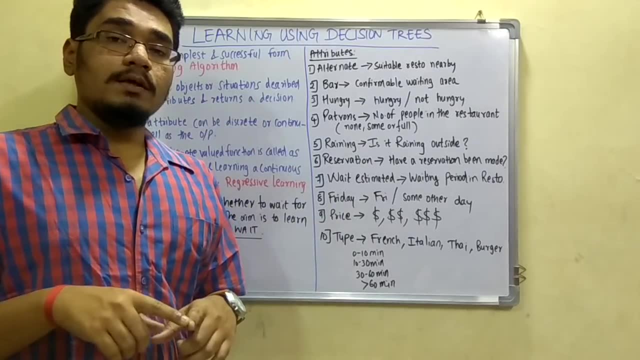 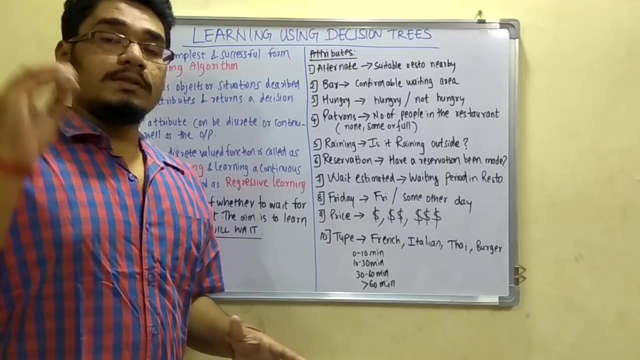 dish, or the Thai one, or the burger one. so for constructing the decision tree, we only consider till the seven attributes rest. all attributes we list out in a table. so that table is a big table consisting of 12 rows as well as the 12 columns. so let us see how this examples. 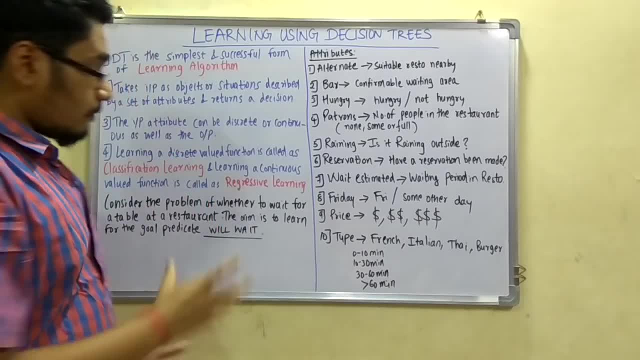 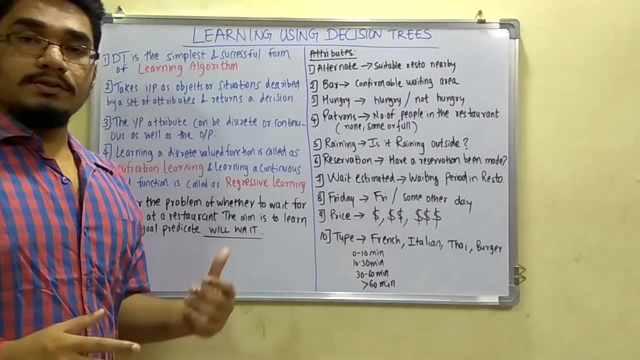 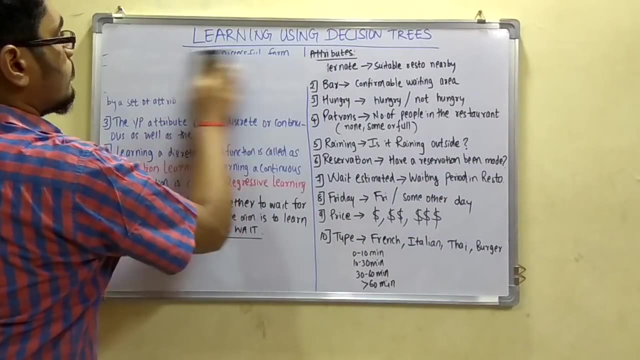 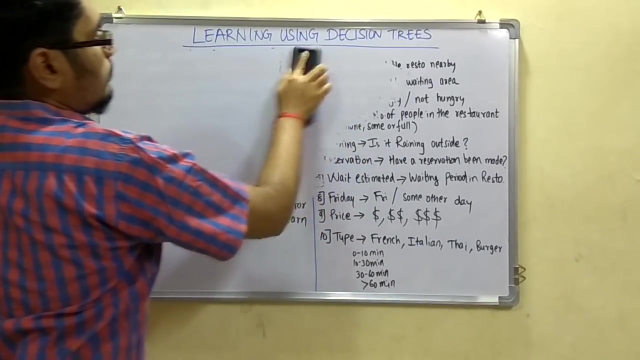 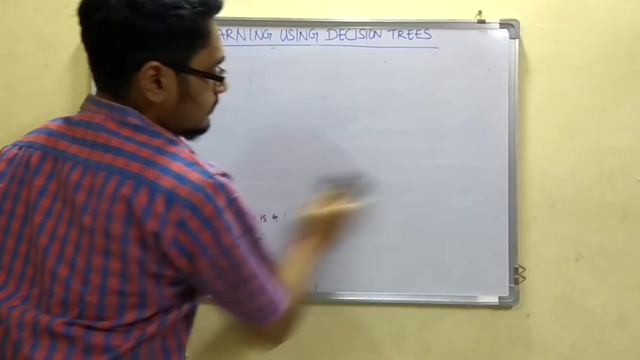 of each and every case is done and whether the robot will estimate for the weight condition. so it is, draw the table for the decision tree item or not. let us learn, basically, the decision trees drawn with the help of this table. so it is, table is the backbone of the entire decision tree. so to consider this, you have to consider. 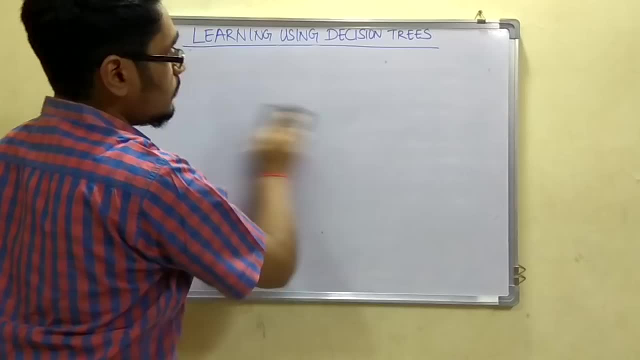 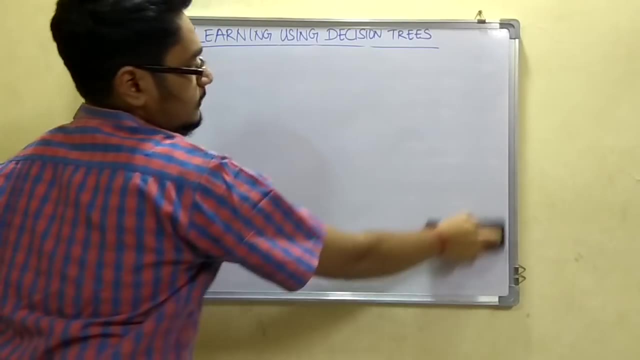 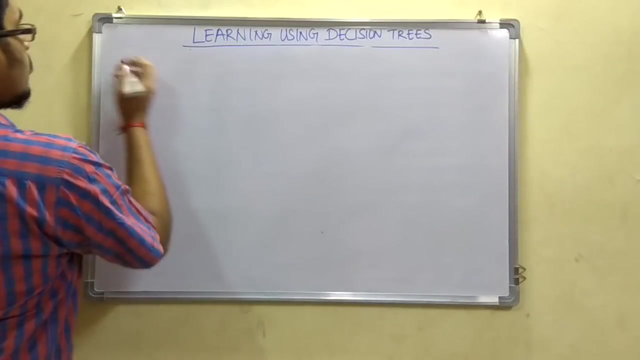 certain examples. that examples can be only of few values or few cases, but in this I'll consider 12 of the individual and independent cases. so let us see what consists of and how to fill this values. so first of all, we have this example means we have taken 12 examples will name it as x1, x2, x3, x4, x5, x6, x7, x8, x9, x10, x11. 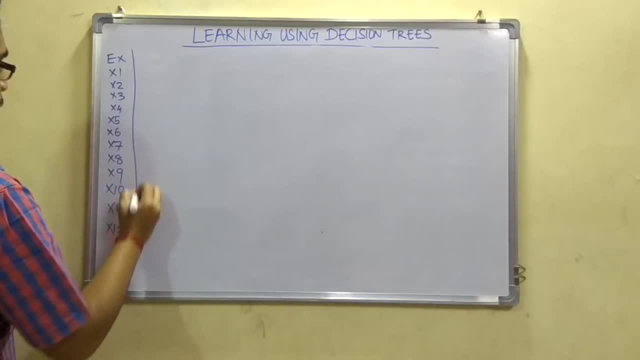 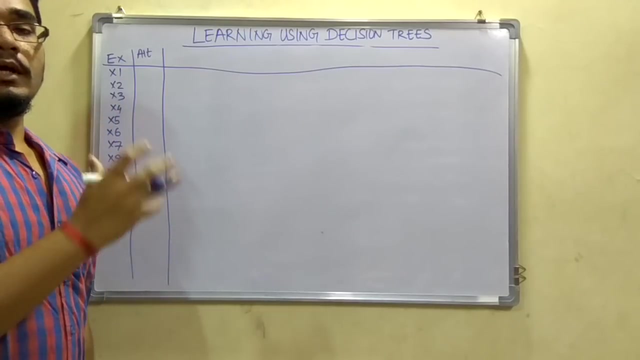 and x12. so here are the 12 examples. next is the alternate that, whether there is a alternate area or not, so let us draw. this will give the values to each of these columns, or more precisely, the attributes as the true or false, the Boolean values we prefer. 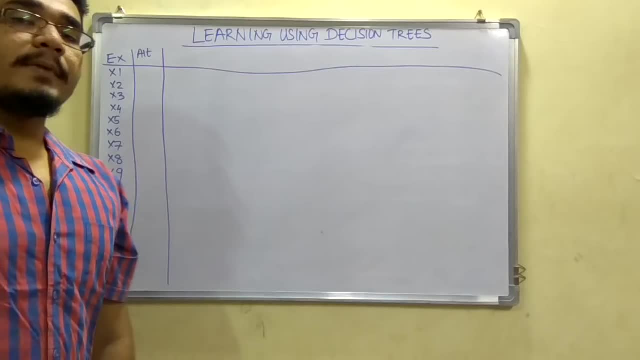 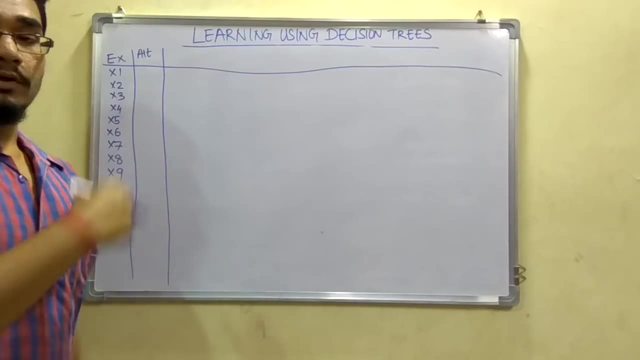 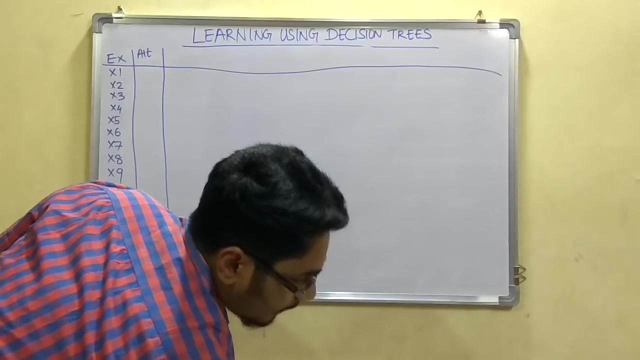 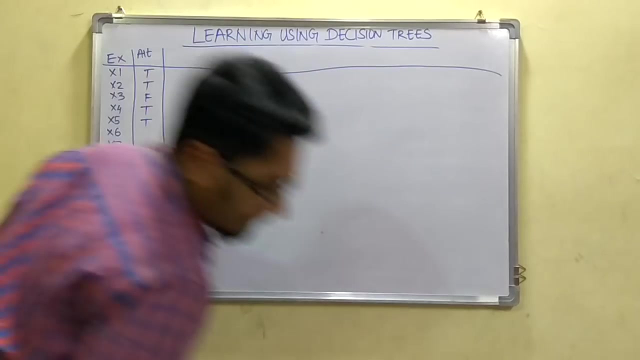 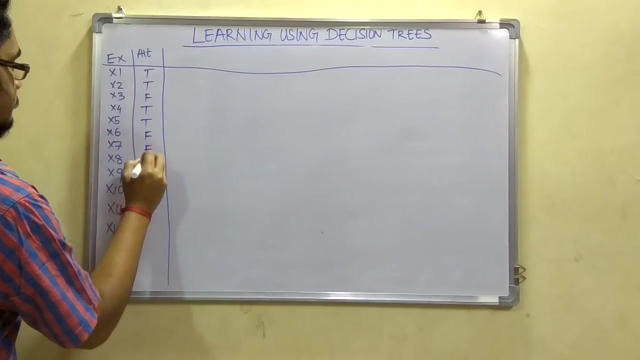 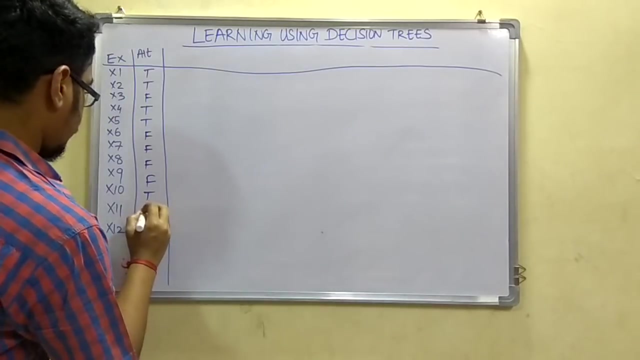 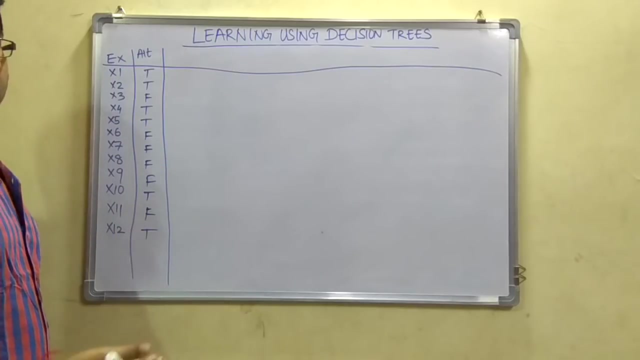 in using the decision trees. so we give some randomized Boolean values like true or false in some manner. so I have made a pattern for this alternate value so that I am going to directly write over here. so it is TT, FTT, TT, FTT, triple TFT. so this values are random. you can take any of this can, interchange, you can. 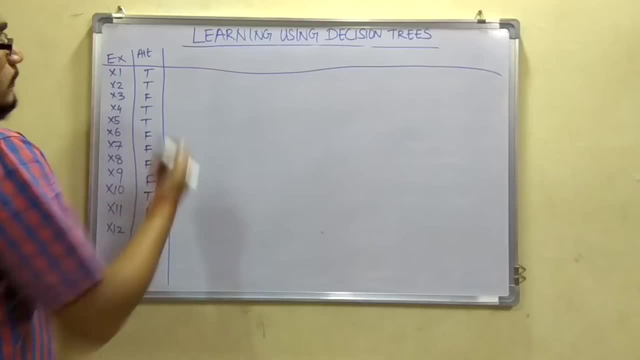 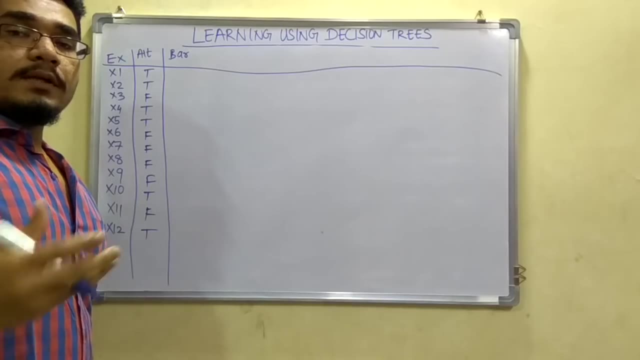 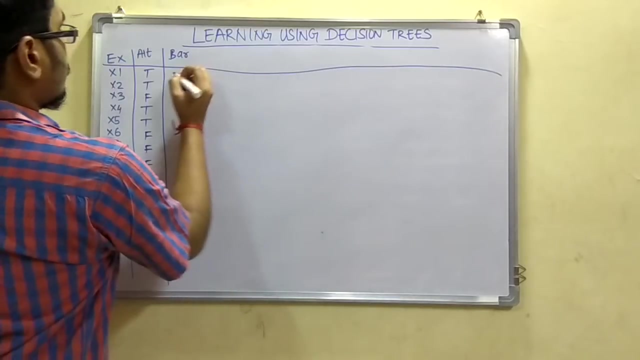 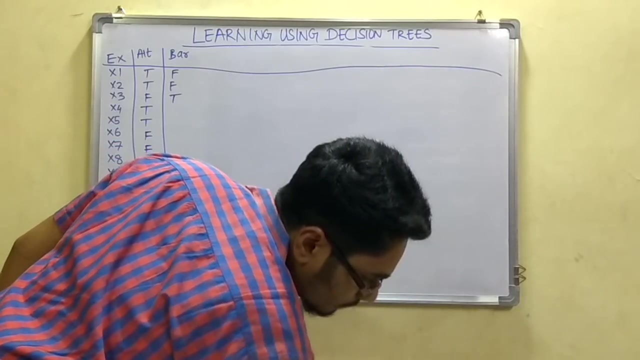 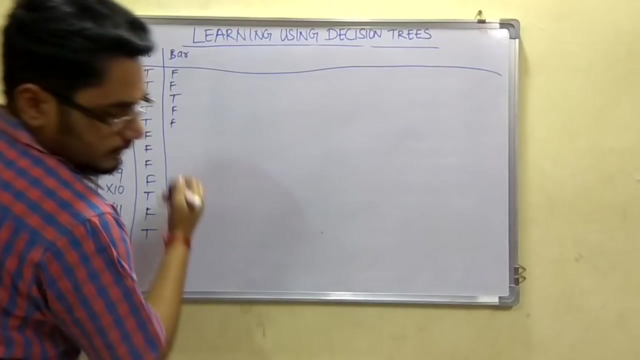 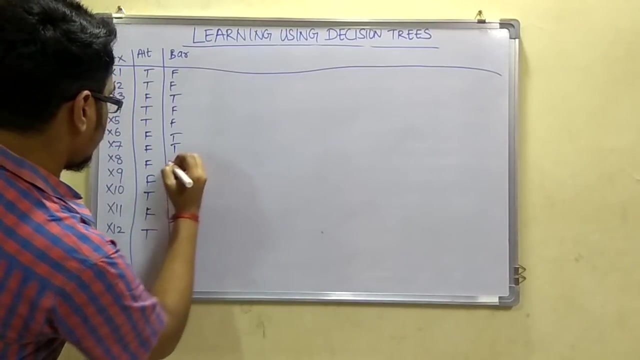 randomize it and can try for more examples. so next one is the bar that whether they have to wait for a particular period of time in a confirmable area, so that also it's randomized. so I have made a certain set. it is FFT, FFTT, FTT, FT. 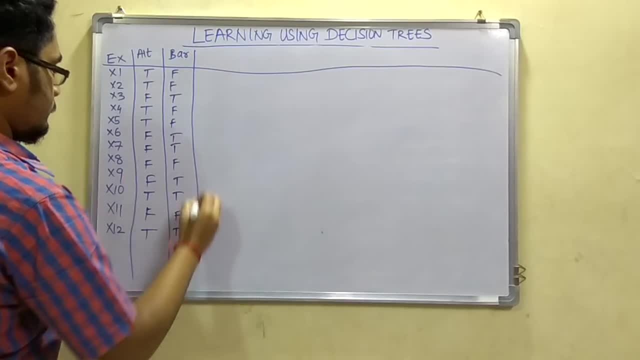 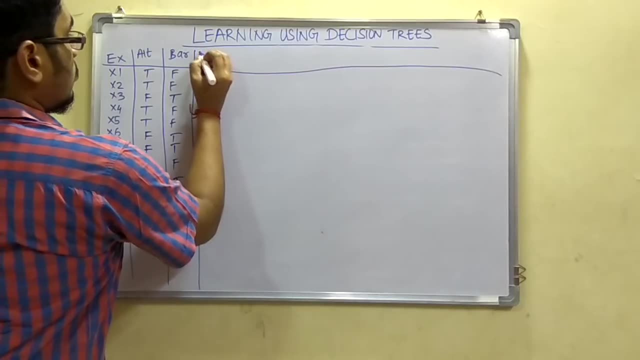 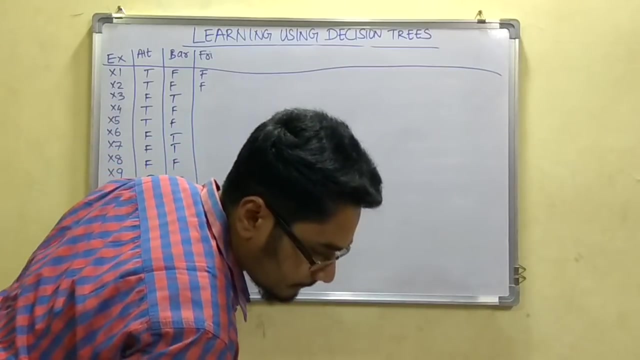 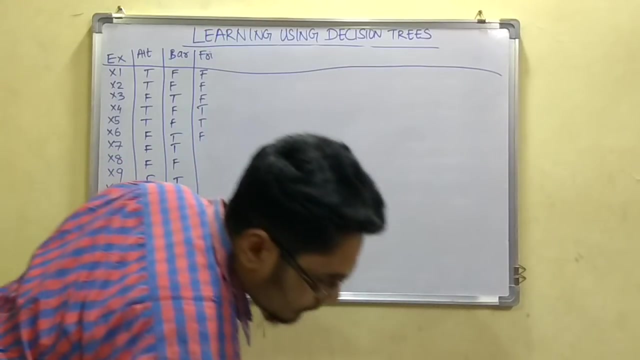 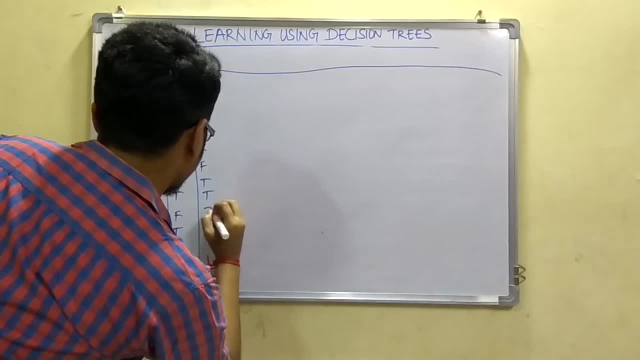 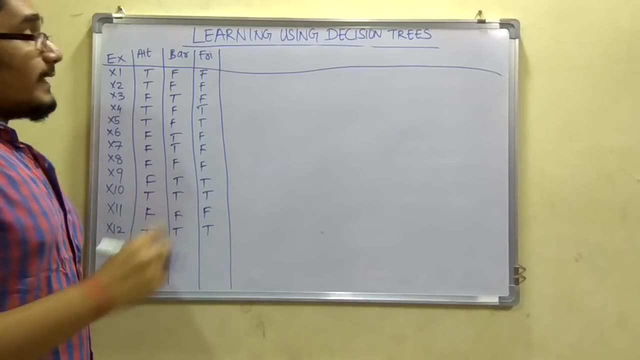 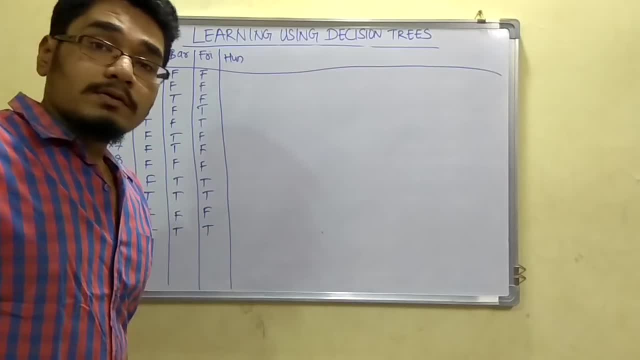 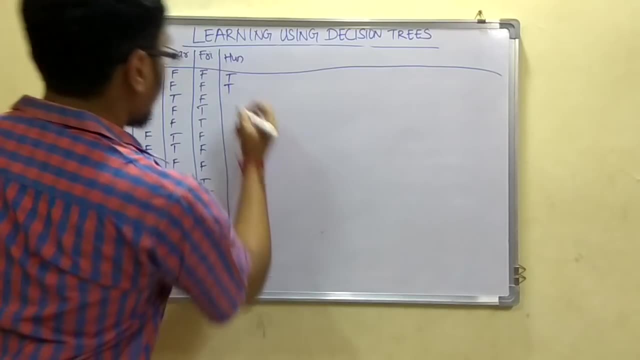 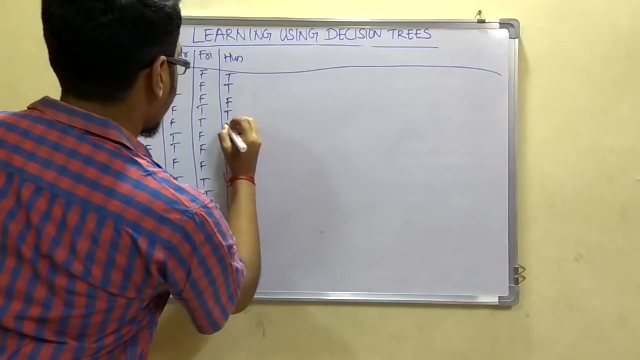 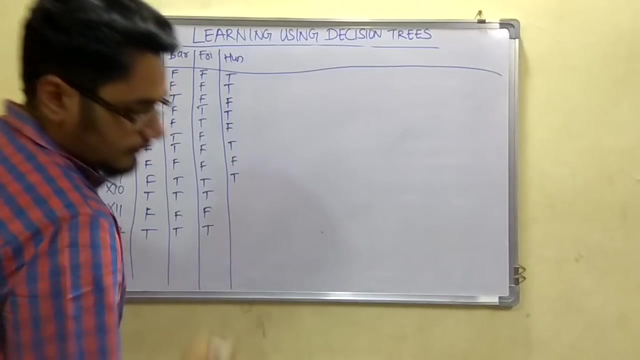 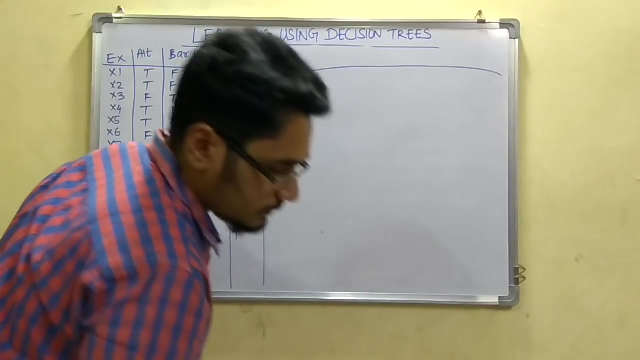 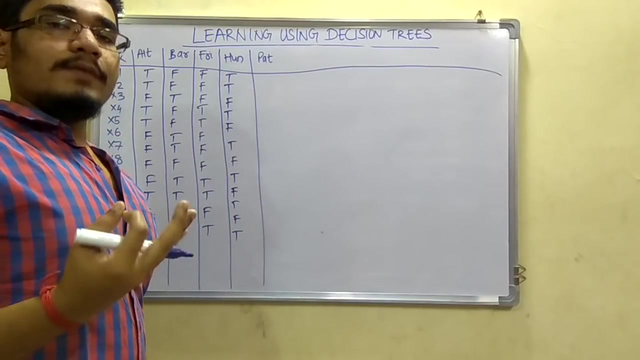 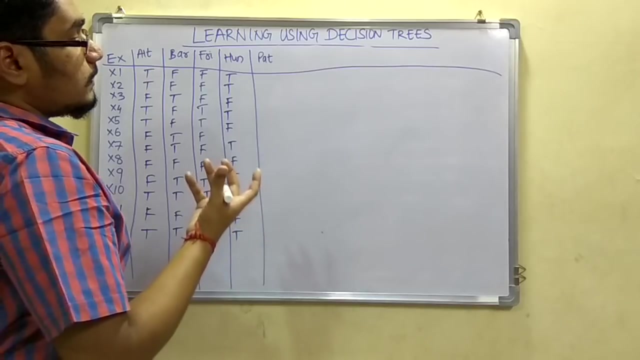 hungry attribute whether the patrons are hungry or not. so for that we have TTT, FFT, then FT, FT, FT, FT. next is the patrons. so the patrons value cannot be true or false. it has got three values, that is, sum or full or none. so we will write it in a denotation form. like for sum it will. 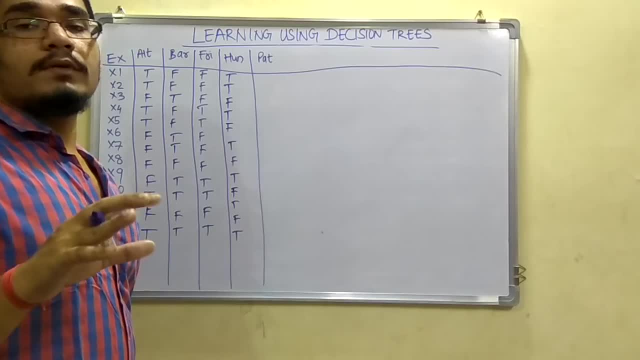 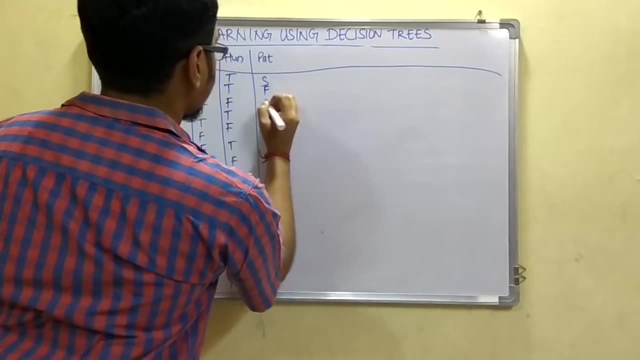 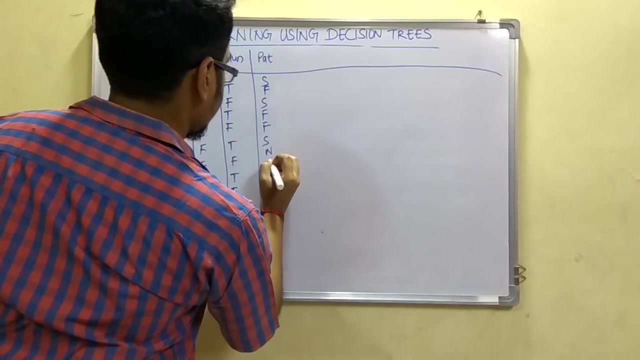 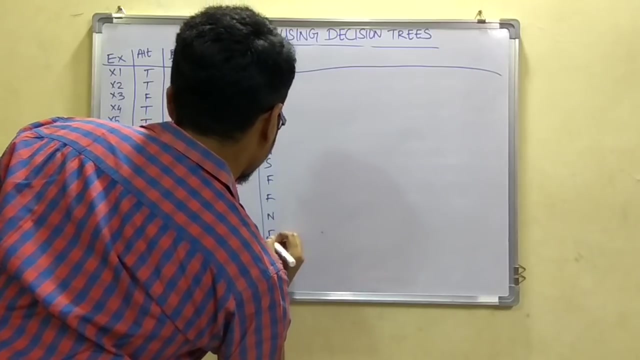 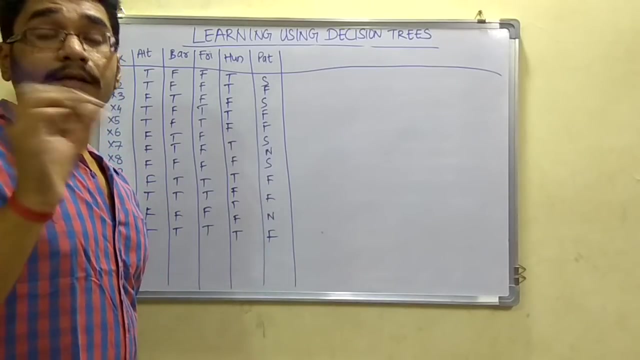 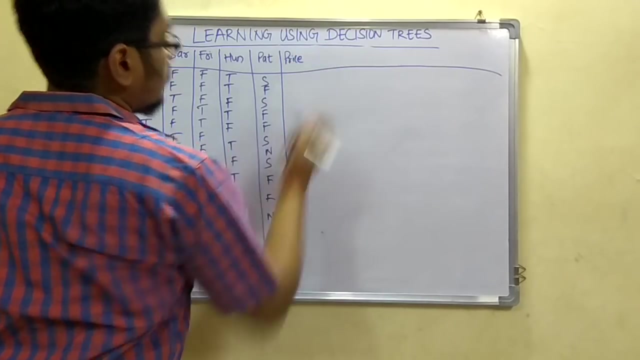 be S, for none in will be N and for full it will be F, so it is S, F S, F, F S and S- Monday and F. next is the price category. we had three types of price, that is, single dollar, two dollars and three dollars. so that price would be coming here and it. 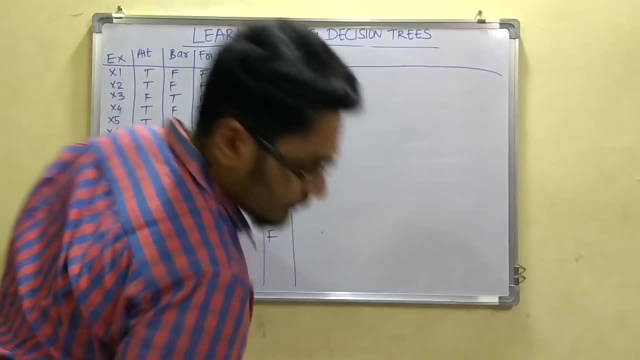 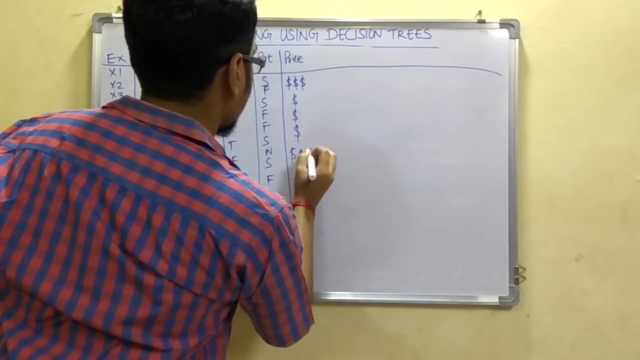 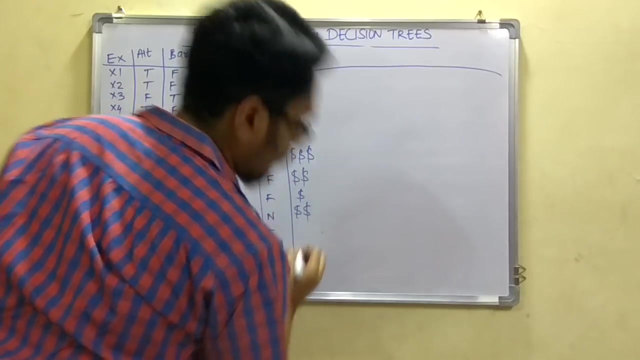 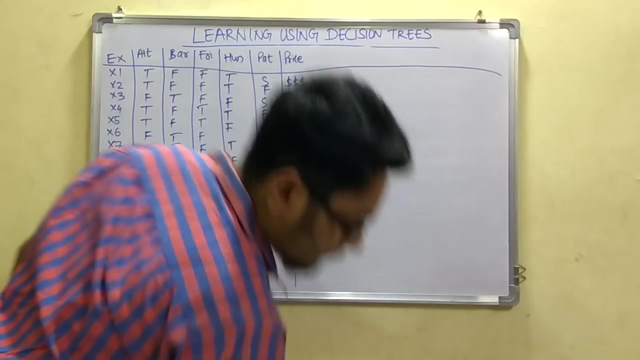 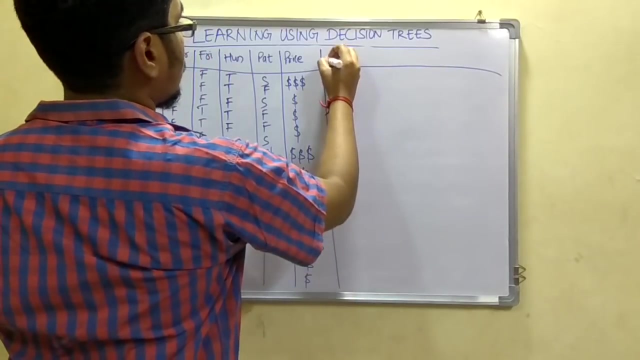 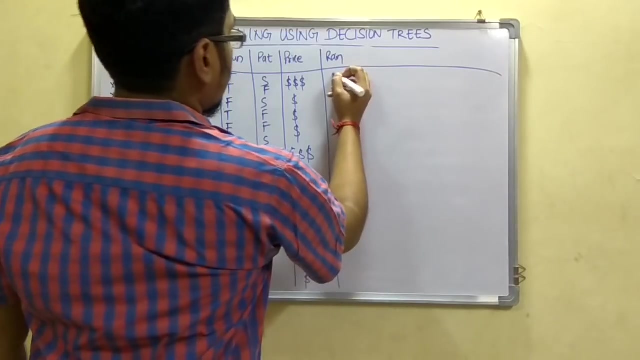 is three times dollar, then single dollar, single dollar, single dollar and three times dollar. two times dollar, then a single dollar, then two times dollar, then single dollar, three times dollar and single dollar. next is whether it is raining or not. raining means whether it is a summer, winter or fall, so it is F. 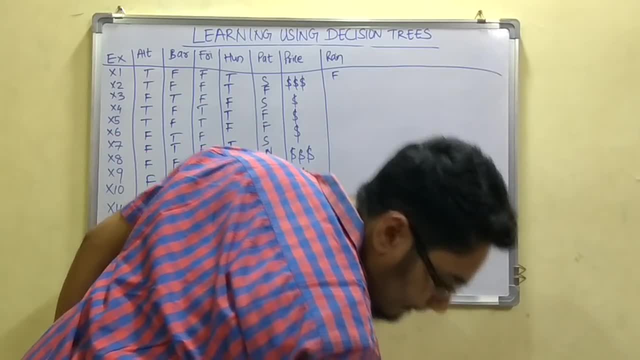 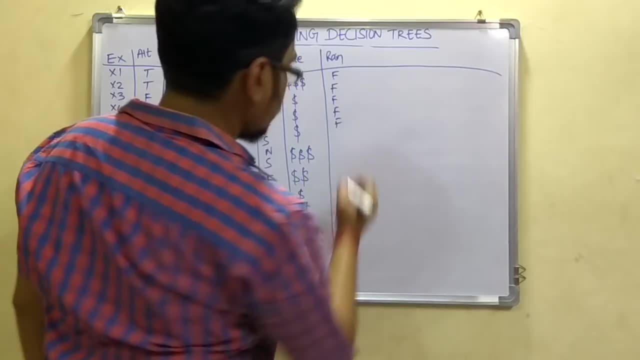 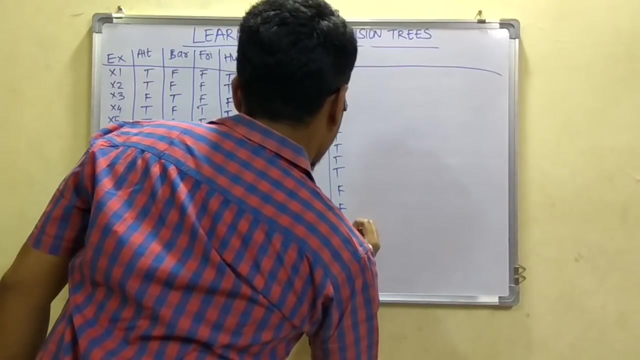 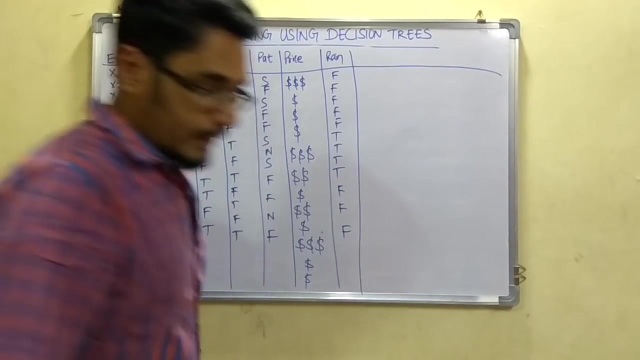 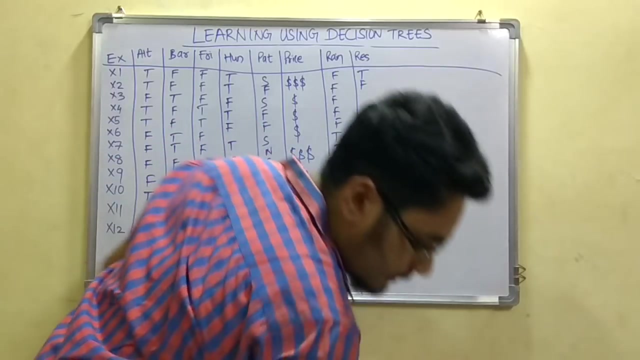 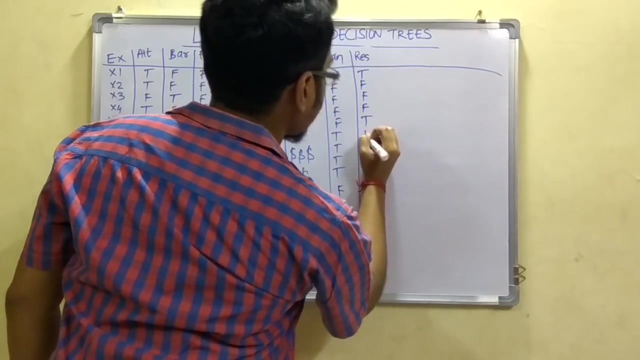 F, it is 5 times F, and it is 4 times T and it is F, F, F. next is whether it is a reservation has been made or not. so for that we have R? E S and it takes T, F, F, F and T, T and F, T and. 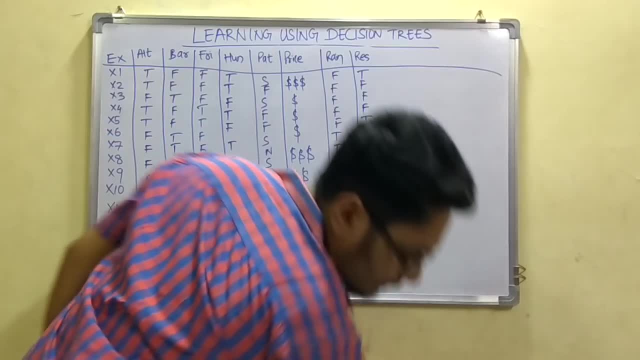 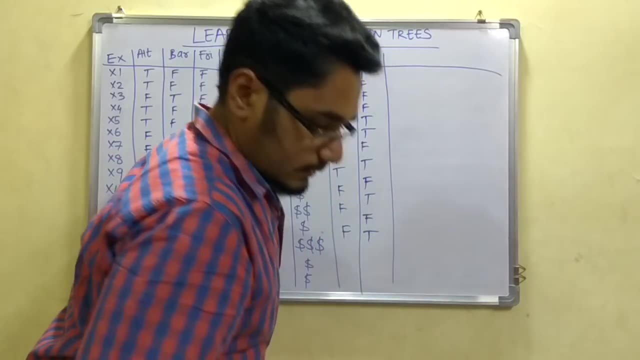 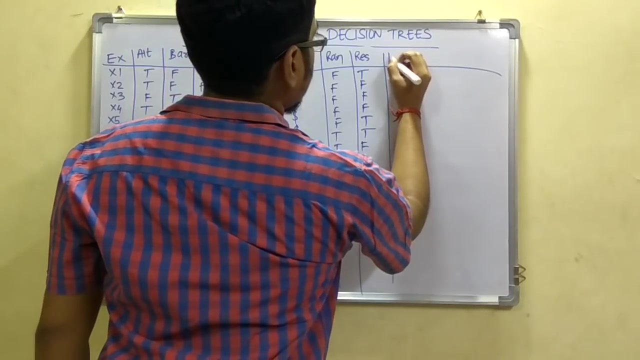 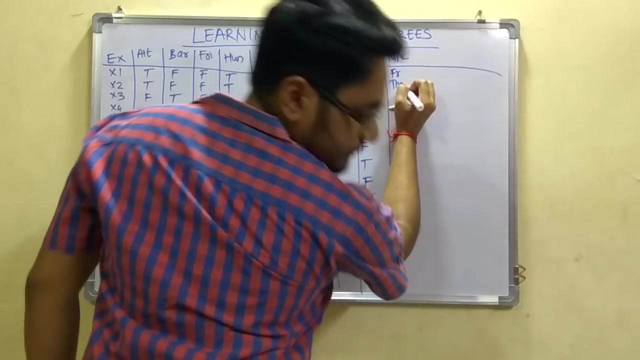 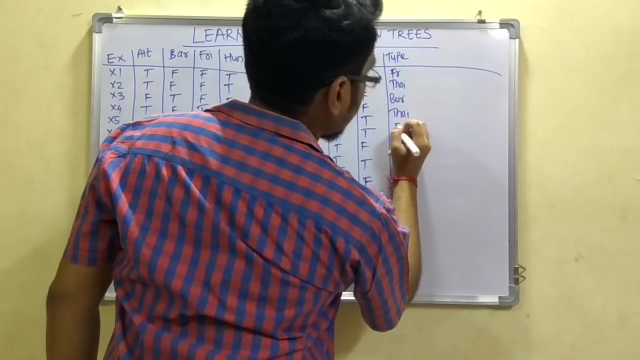 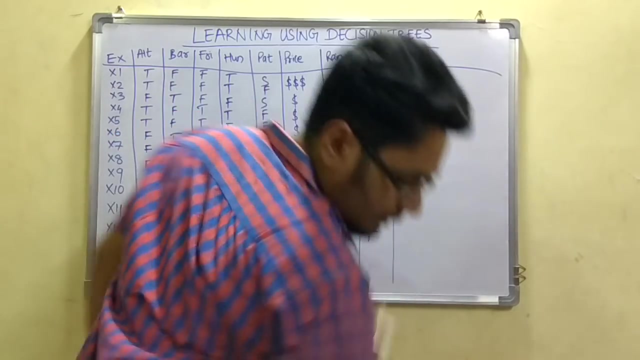 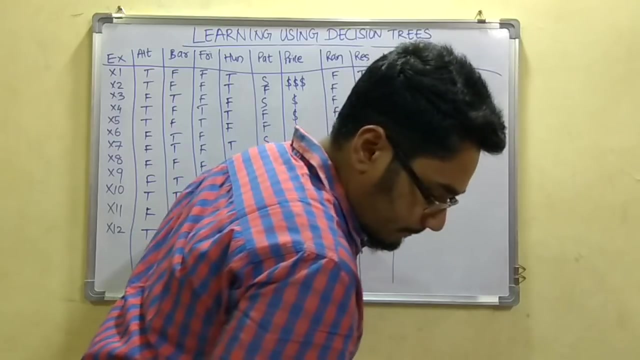 F, T, F, F, T, F, T. next is the type of food, whether it is an Italian, French or burger. so the type of food, that is, the French, Thai one, the burger, again, the Thai comes, then French, then Italian. I am using the notations, so a space constraint is there, and that's. I am denoting it with smaller notation. 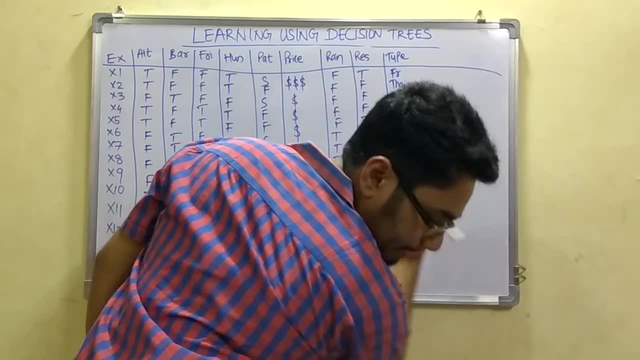 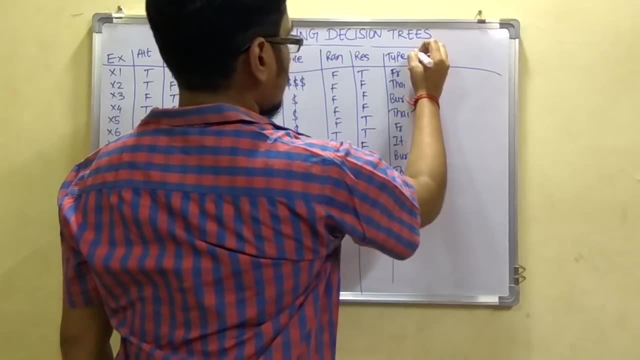 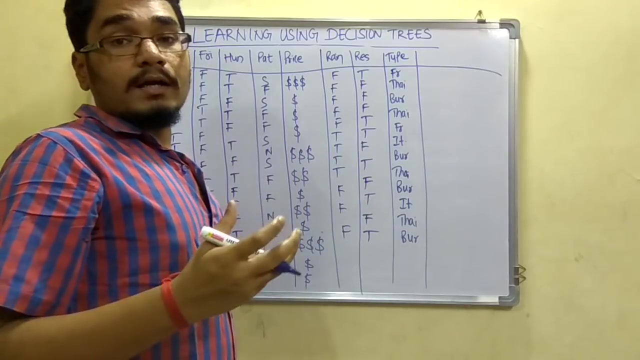 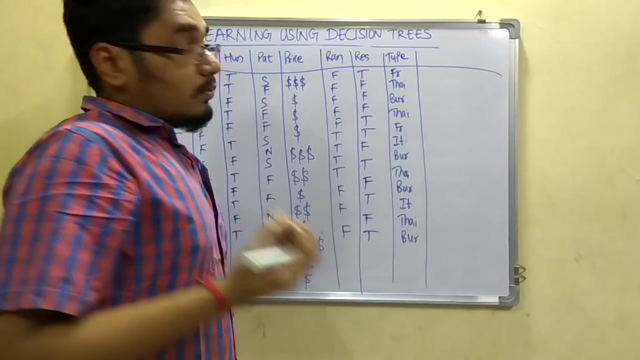 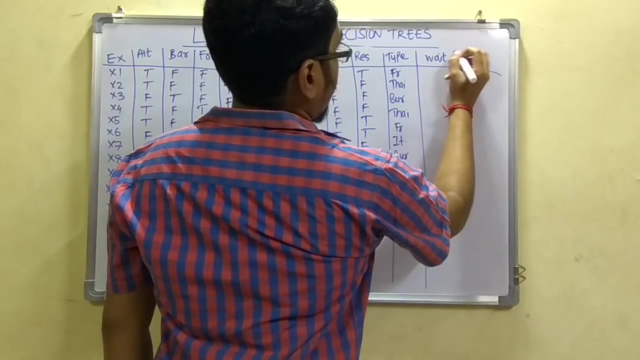 then it is Thai, then Burger, then Italian, then Thai and Burger. so now the final. that is the aim of our decision tree, that is, to consider whether the pattern has to wait or not. so our final column would be the aim column, consisting of the estimation, the weight estimation. so this will 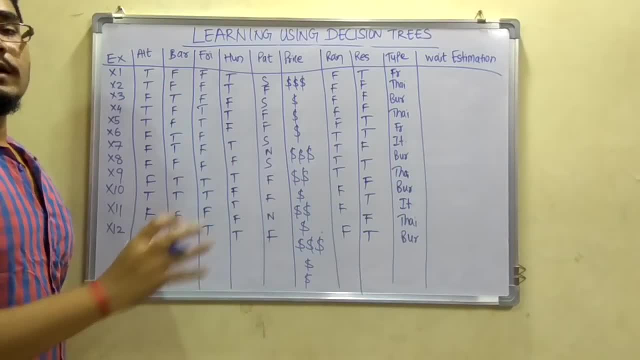 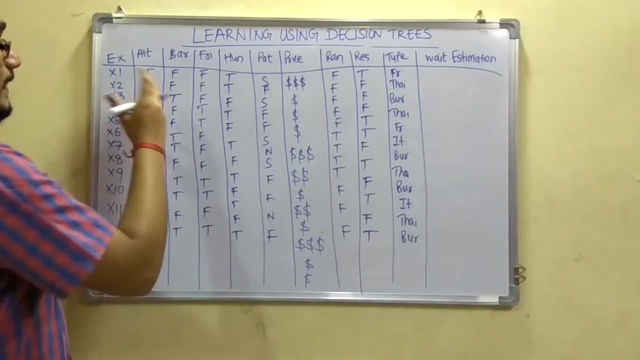 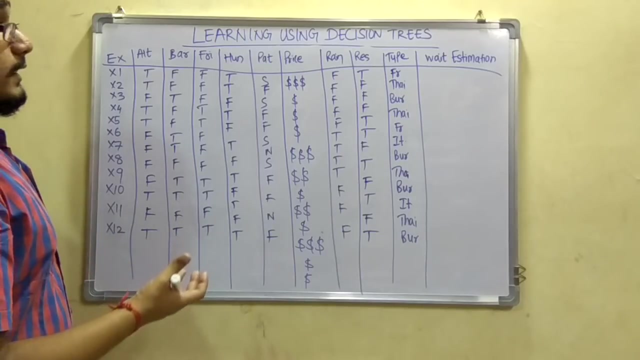 depend upon the entire rest of the attributes. so whether, in the first example, if there is an alternate restaurant is available nearby, and if that restaurant doesn't have a bar, that is the waiting area, and if it is not a Friday and if the patrons are hungry and the price is somewhat costly, and if it 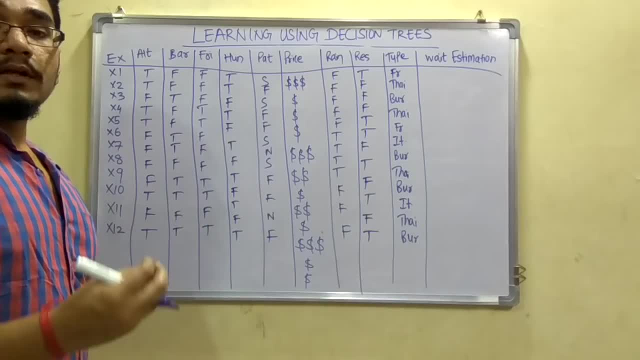 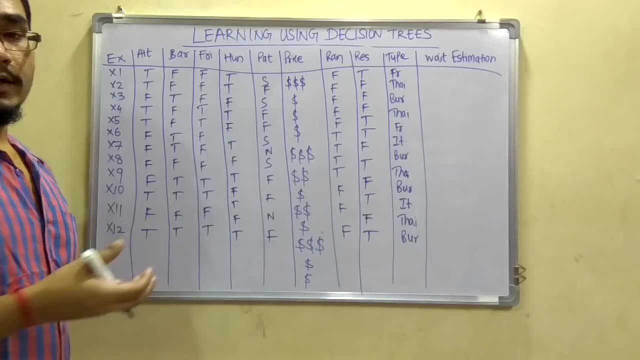 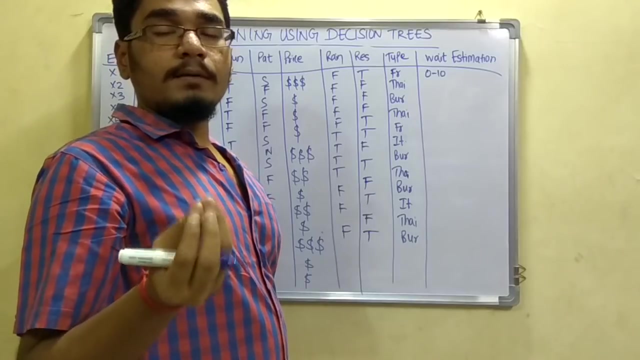 is not draining and there is a suitable- and they've already made a reservation for that- and the French type is there for food, then the weight estimation in this case could be 0 to 10 minutes, that is, it will be waiting for a particular period of. 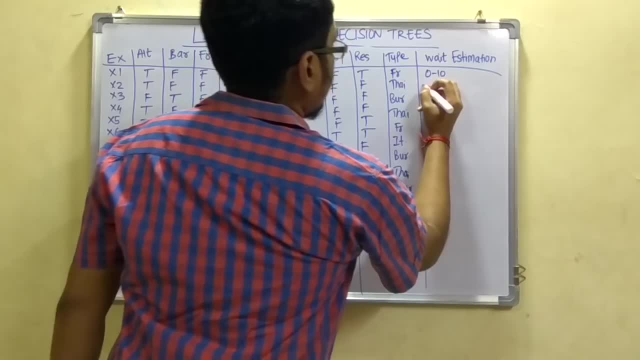 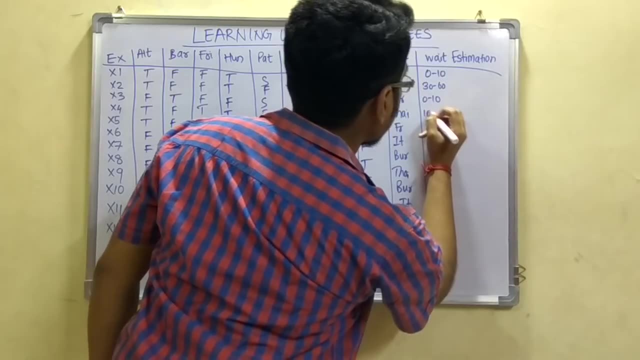 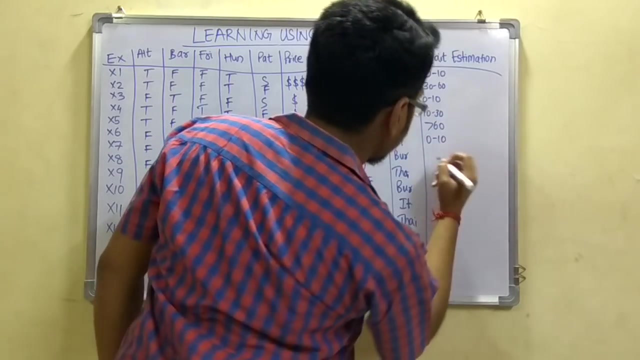 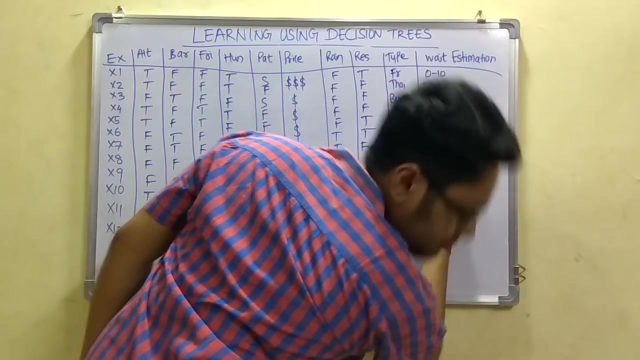 time. so likewise I have drawn a certain set, that is 30 to 60 and 0 to 10 and 10 to 30 more than 60, 0 to 10, 0 to 10 more than 60 and 10 to 30, then 0 to 10 and 30. 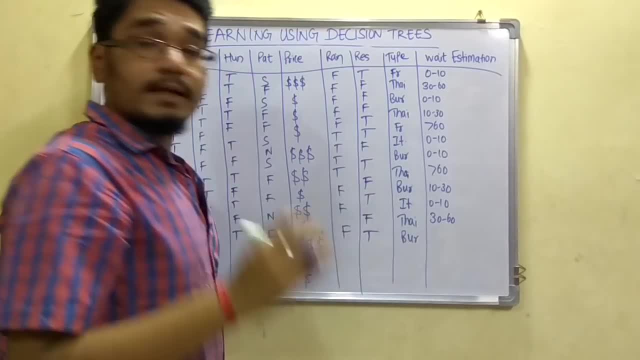 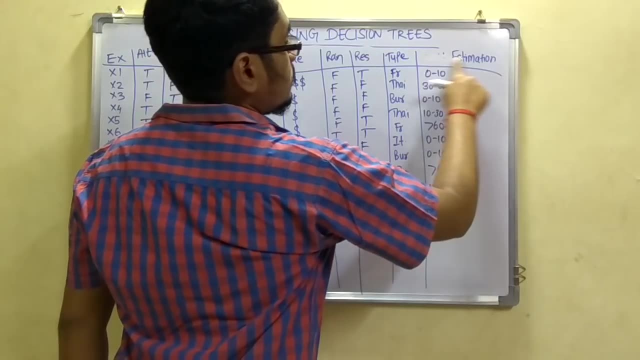 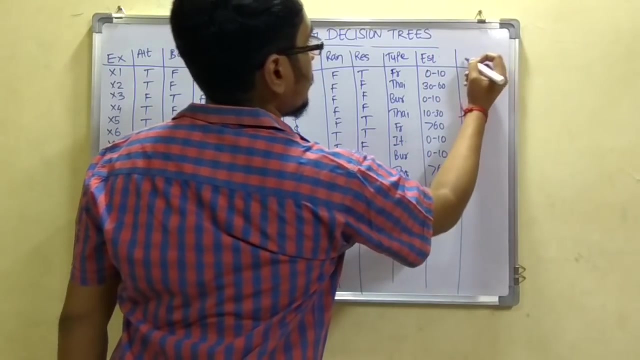 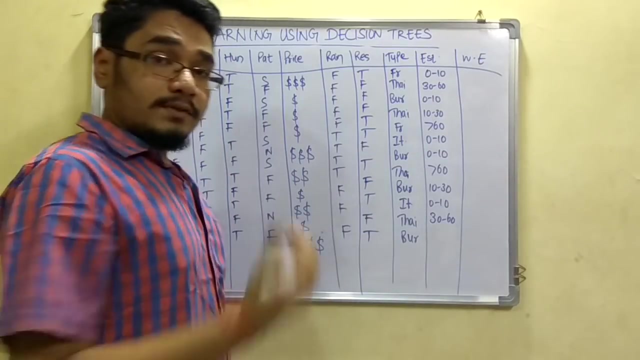 to 60. now, after this estimation of the time, there will be the estimated wait time and this is not the read estimation. this is the estimated time, that is the ESD, and one more column will be coming. that is the weight estimation, that is the w? e column, so that column is the final column in. 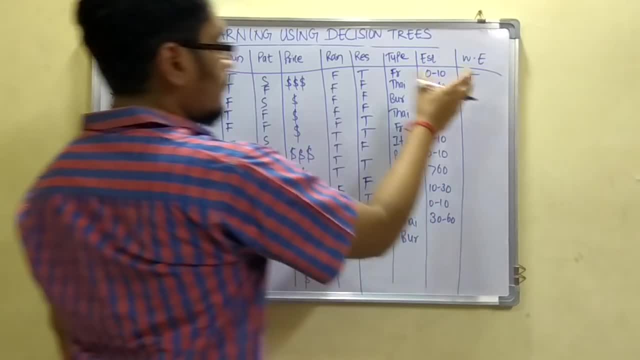 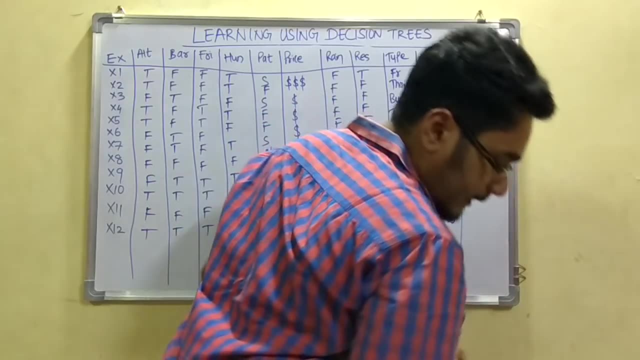 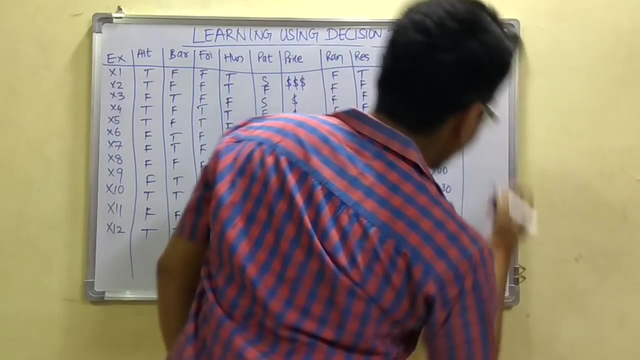 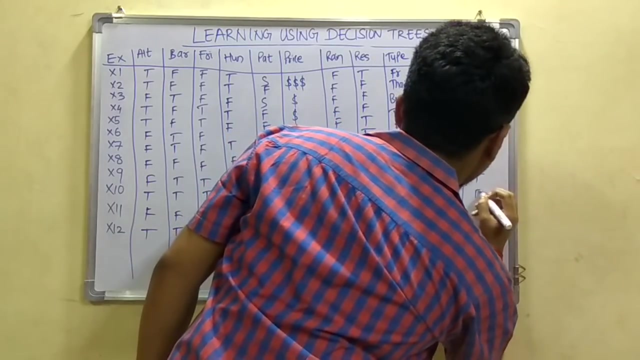 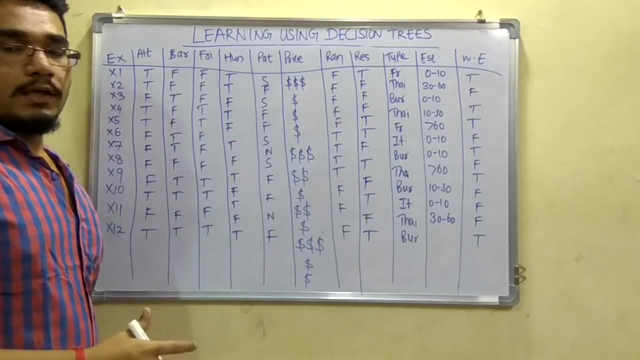 the division tree. so for that now, this values are all dependent upon the previous columns of the previous items. So it would be tf, tf, tf, td and ft, ft, and it is 3 times f and 1t. So this is the table of the decision tree. So now, based on this table, we would 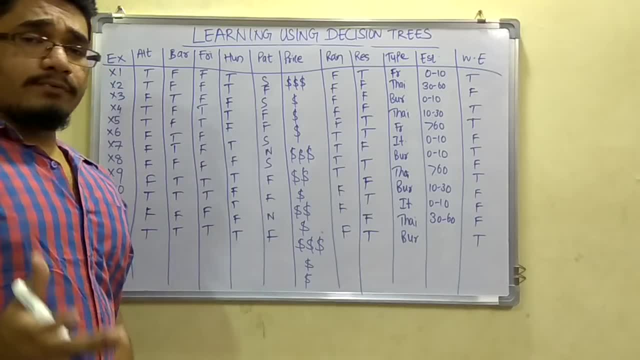 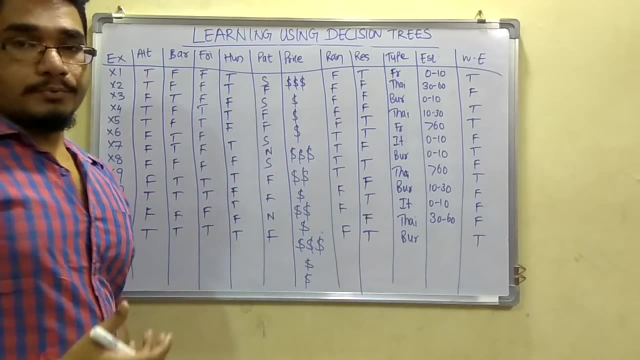 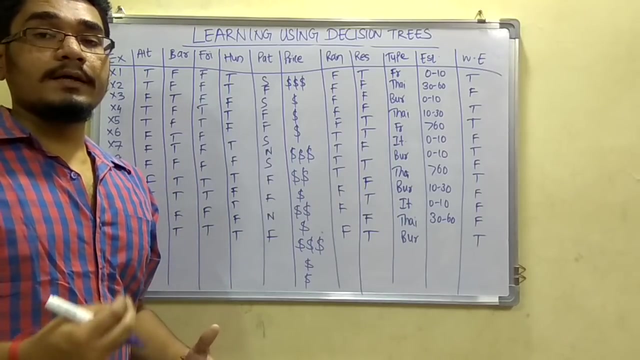 be constructing the final decision tree. So for that final decision tree we would not be considering the type as well as the price attribute for considering. So it can also be considered, but then it would become more complex and it would be taking more memory. 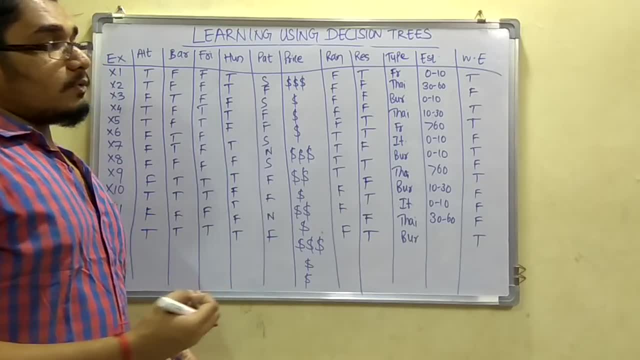 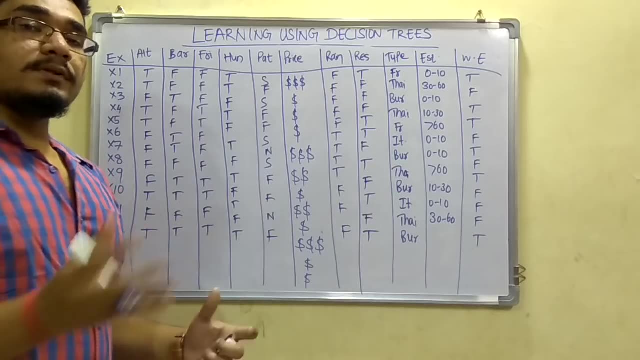 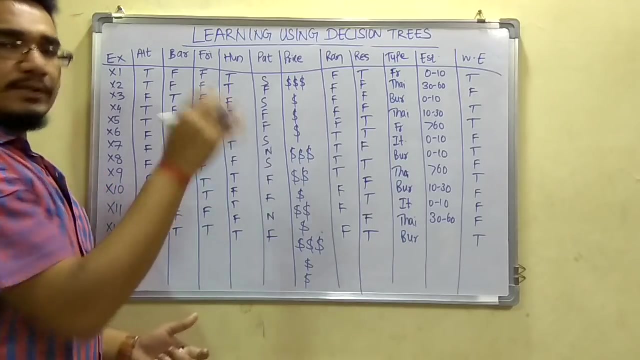 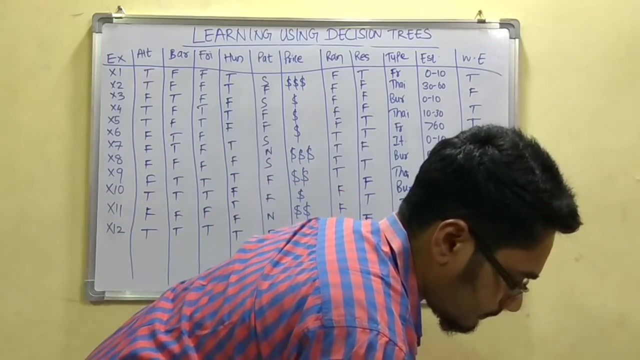 in the computer space- computer memory in fact. So to avoid those complications, we will construct it in a simpler manner, A simple small decision tree where user can easily understand it. So after this we will be considering our final decision tree using this table. So let us see how that tree is constructed. 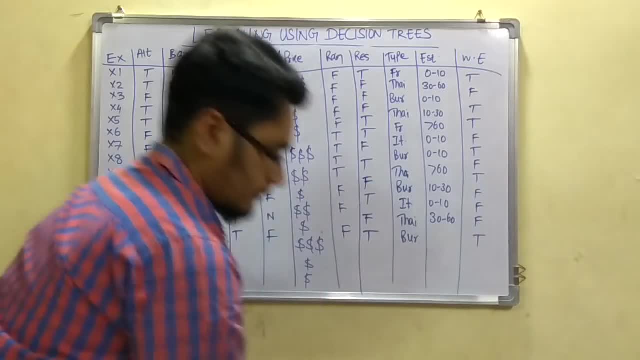 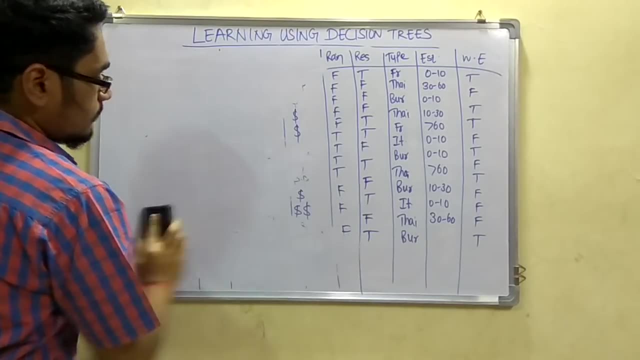 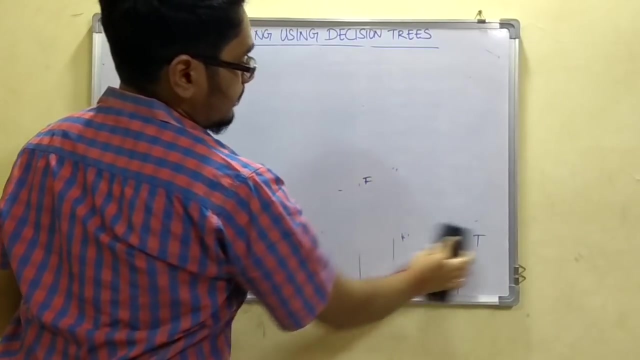 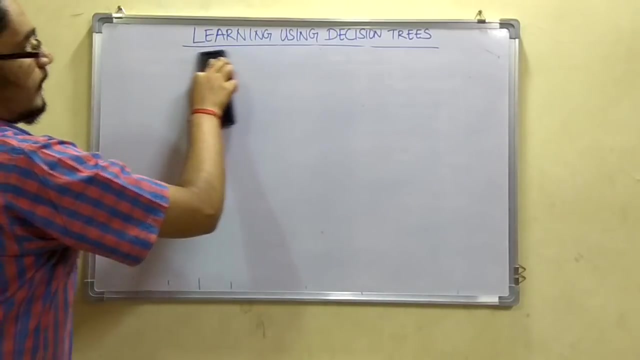 So for that we have to make an estimation. Now there is a space constraint here, So that's why I am rubbing it out, means it's somewhat big, not big actually it is. we have to link it with edges and nodes, So there needs to be much space in this, otherwise it 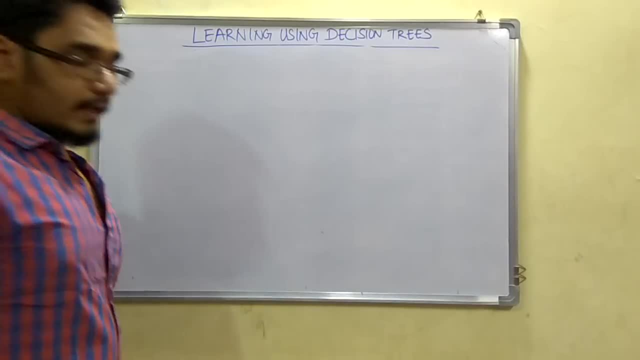 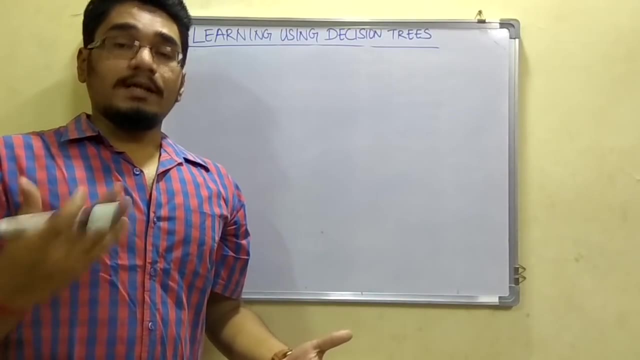 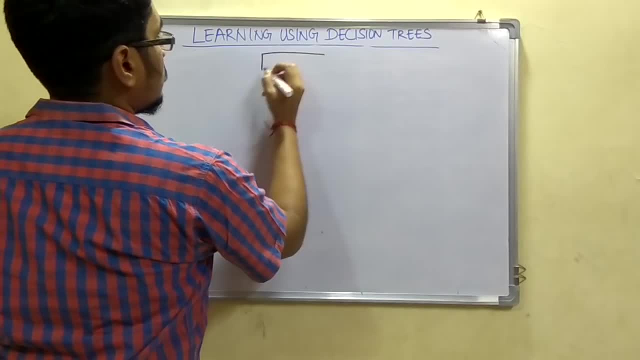 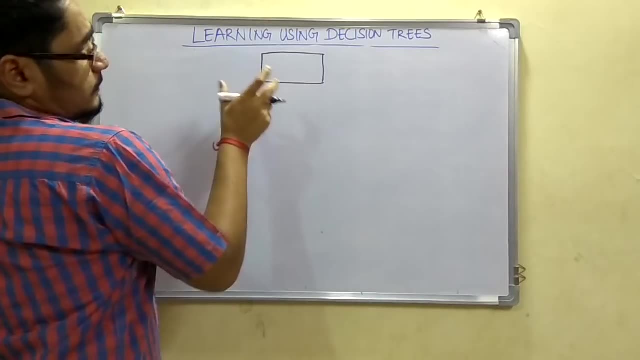 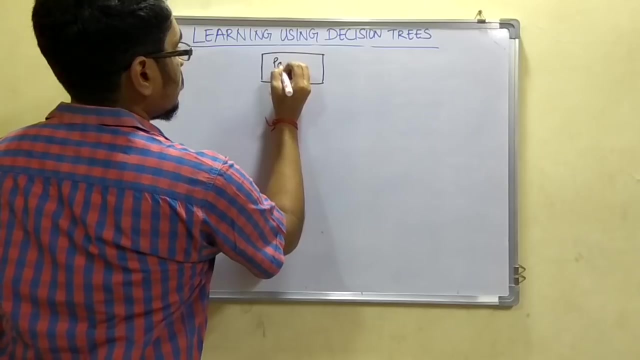 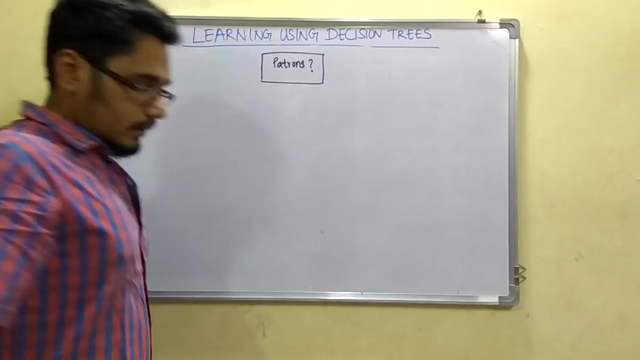 patrons would be the very first node in this decision tree. So decision trees are basically made of this small rectangles or squares and connected with the links as the edges. So it would be patrons and how many patrons, whether it is some full or none. So for that we 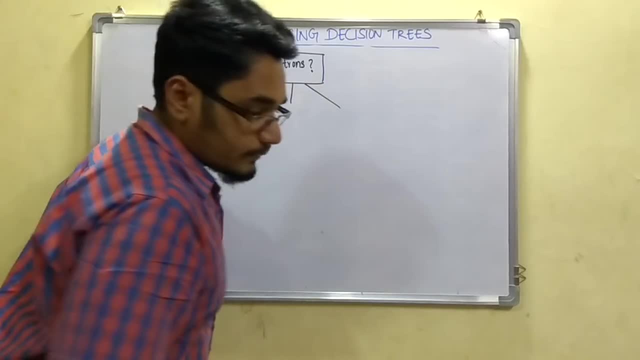 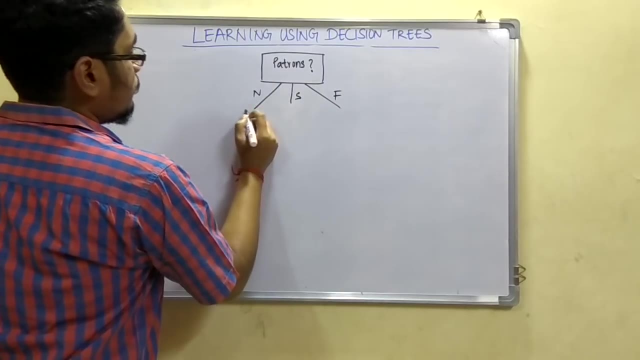 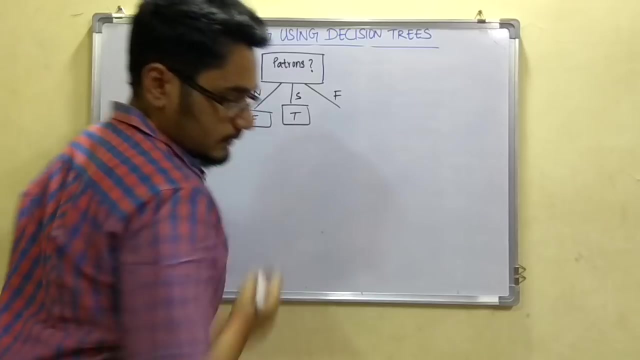 have these three links to that. So n is for none, s is for some, and it is full. Now, if it is none, then it would be false, and if it is s, it is t, and if it is full, then a weight estimate. 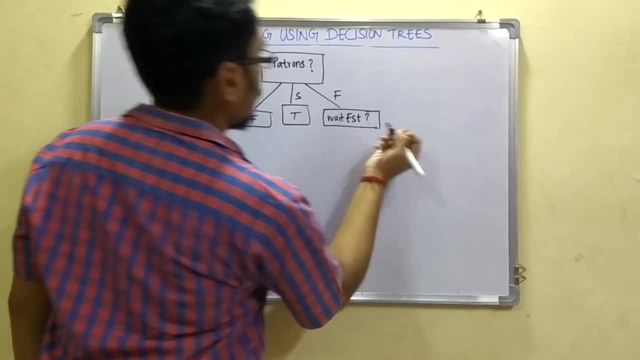 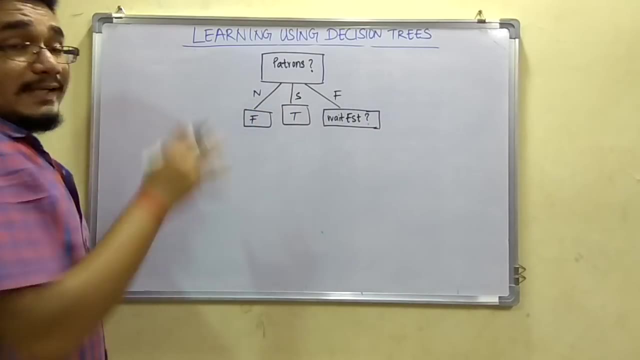 they will wait Now. this final decision tree is called the Poisson's theorem. Poisson's theorem is known as Poisson's theorem and it is used by many tree of this tree ends based upon this F or T whenever the F or T node comes, that 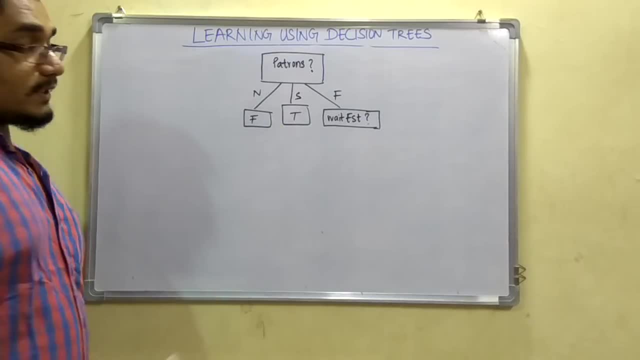 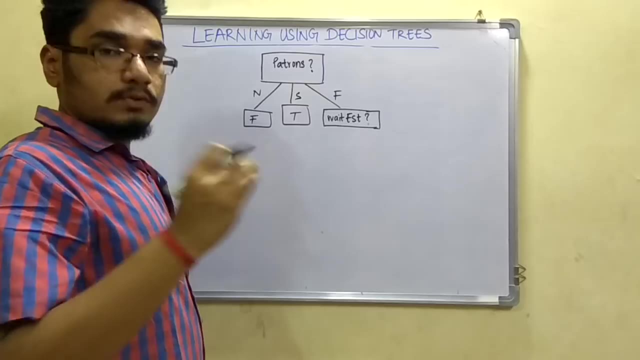 means it cannot be further more expanded. now, the node which can be expanded is the weight estimation node, so we will expand this more. so this weight estimation is of four types, as we said, like 0 to 10, 10 to 30, 30 to 60 and more. 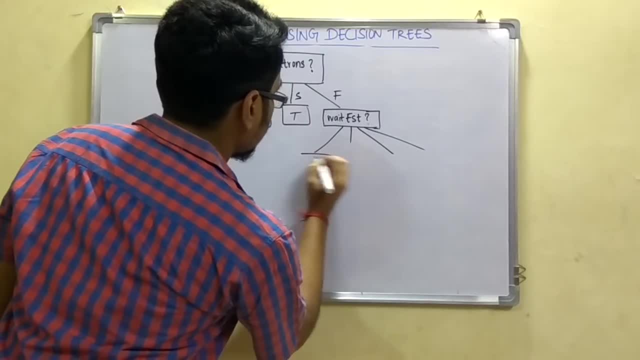 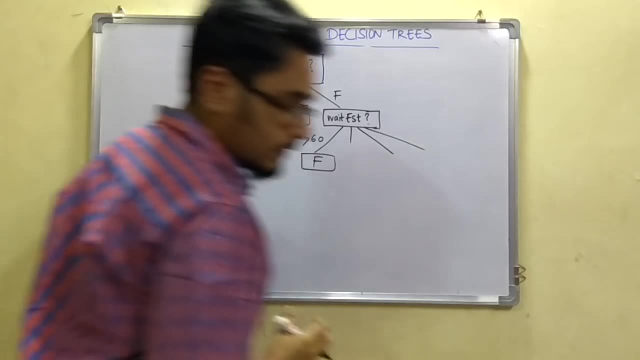 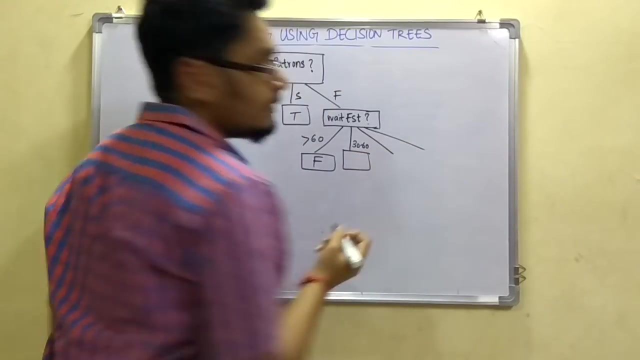 than 60. so we have first more than 60. so for sure the patrons are not going to wait. so F would be considered there and this would be the 30 to 60. if 30 to 60 is the waiting time, then customers would suggest for alternate restaurant. so it 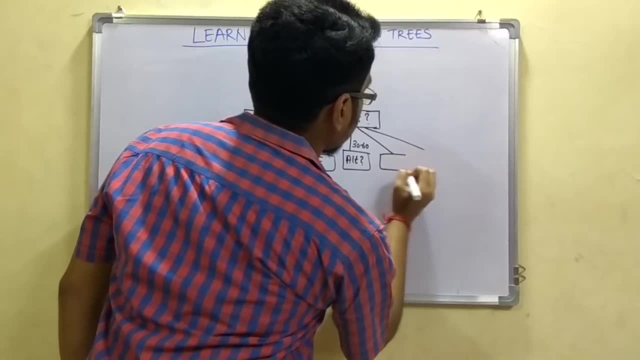 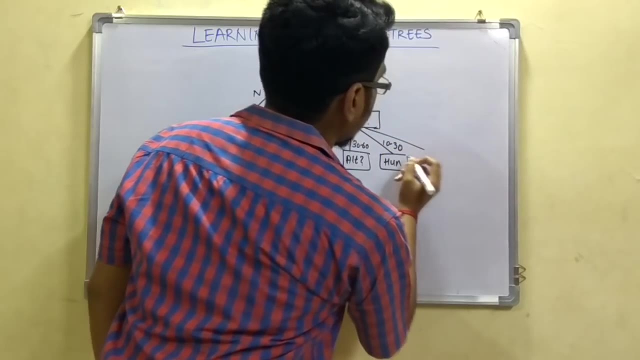 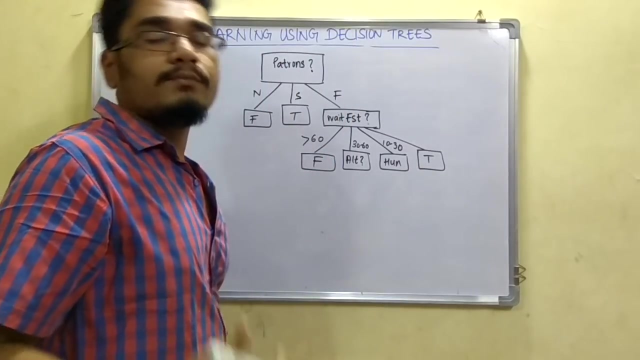 is ALT. next, whether it is the hungry case, whether the patrons are waiting or not, hungry or not, so for that we have 10 to 30 minutes, and if it is 0 to 10 then they would, uh, surely wait for some time and they would enter the restaurant. so it is 0 to 10.. next, 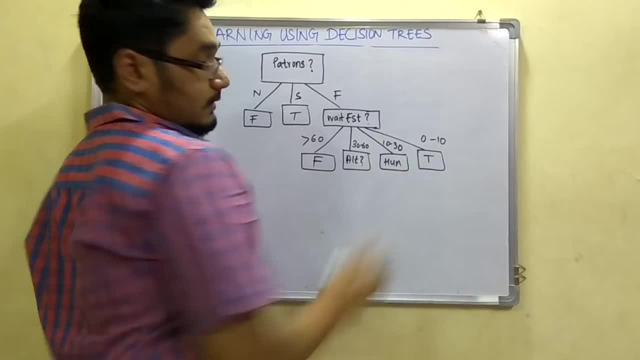 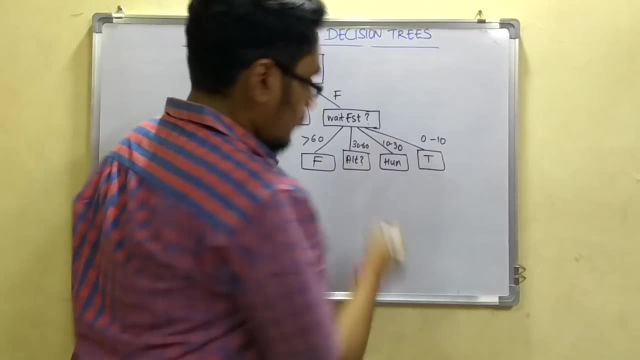 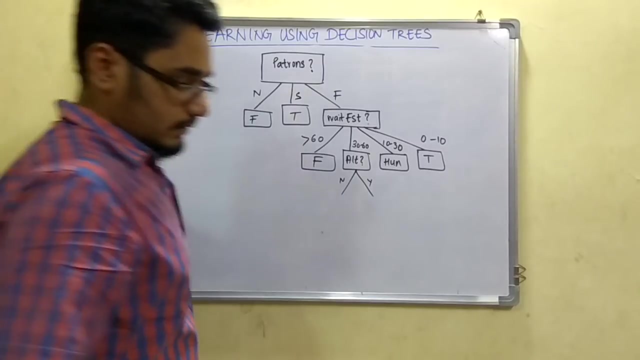 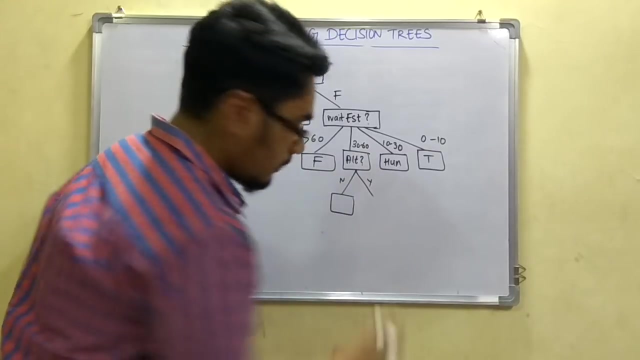 we cannot, furthermore, expand this and this node, so we'll further go deep to this alternative as well as the hungry node. so alternate has two branches, that is, if it is no, or if it is yes. if it is no, or if the alternate restaurants are not available, then whether we have made a 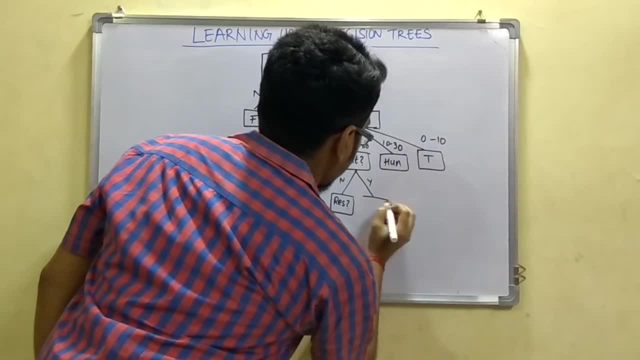 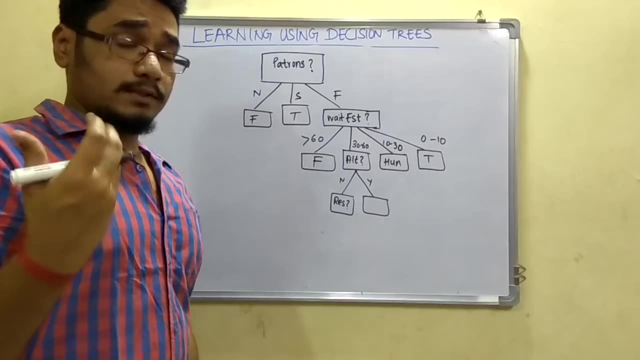 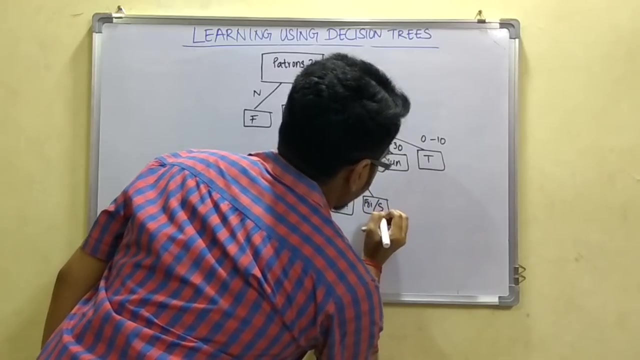 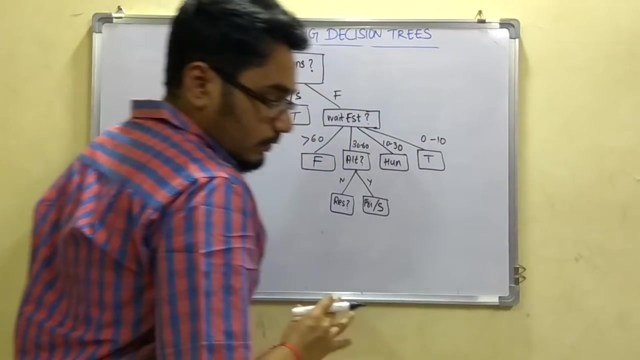 reservation or not? and if it is yes, then if we are entering into that restaurant and if that day is a friday or some other day, so for that we have friday or some other day. as for some other day it can be sunday, saturday or other days of the week. so now this uh restaurant or, sorry, uh the. 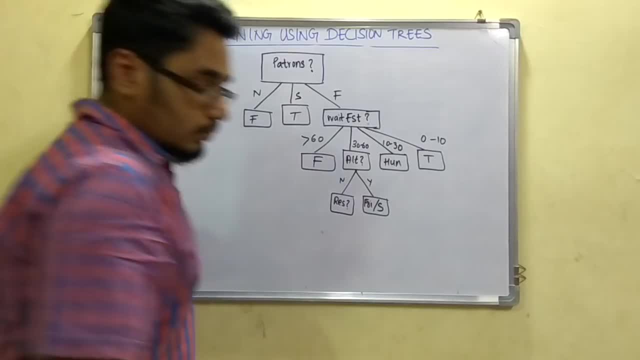 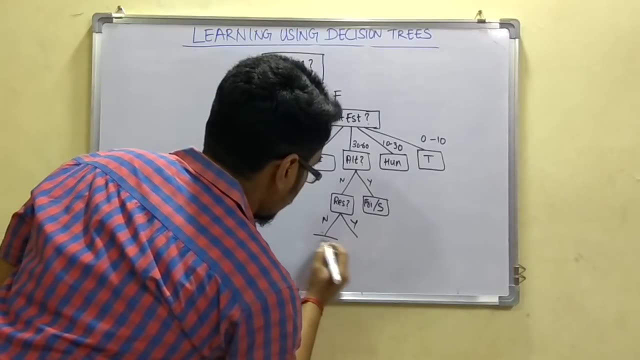 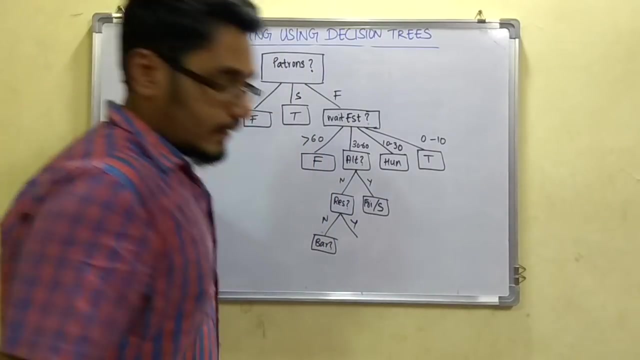 reservation can be further expanded to two: that is the if it is no, or if it is yes. if it is no, here it is the, if it is no, it is false, and then it is true. and as you can see that all this is for a no, or both before and after theеци, when this same jos has been consider available. therefore, 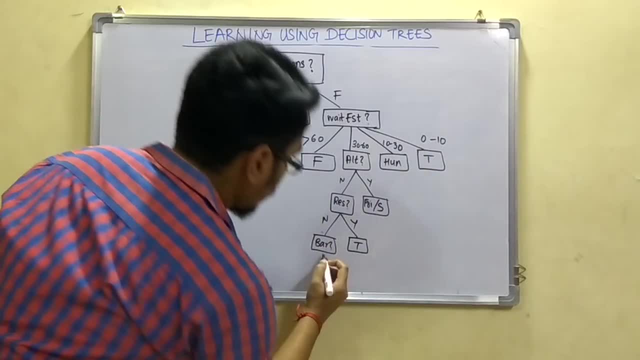 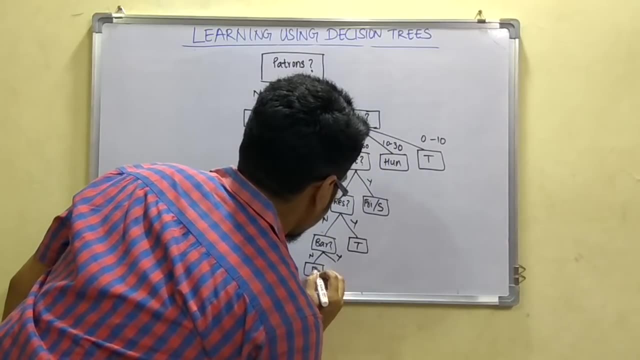 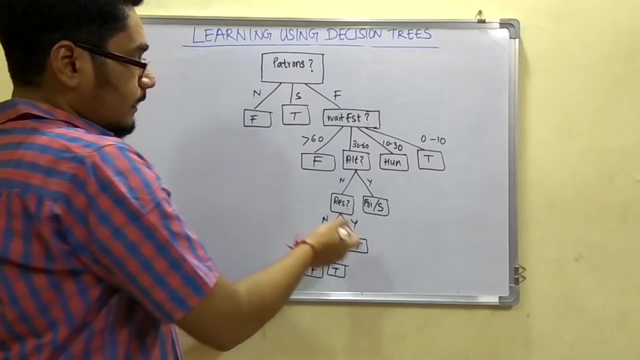 the styles is not same also, for this is the same with some other types, and then that restaurant has a bar that is suitable, uh, confirmable waiting area. so, and it is true, whether it is yes and now Right, be coming to true and for no, it will be coming to false means. that condition is. 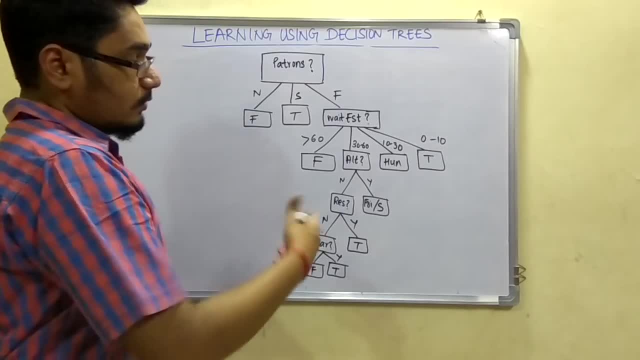 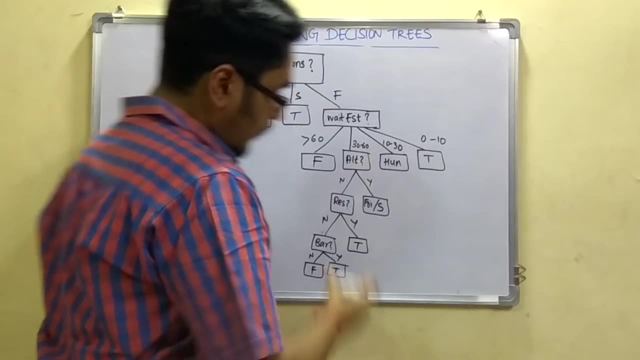 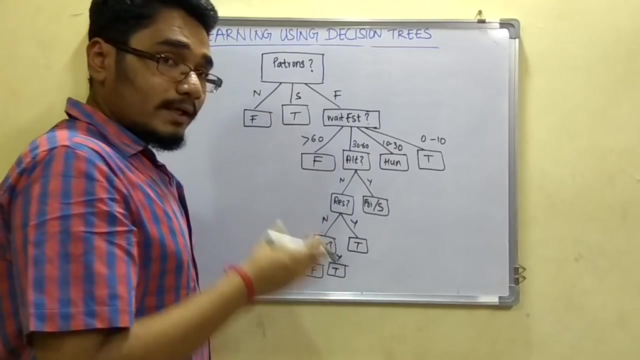 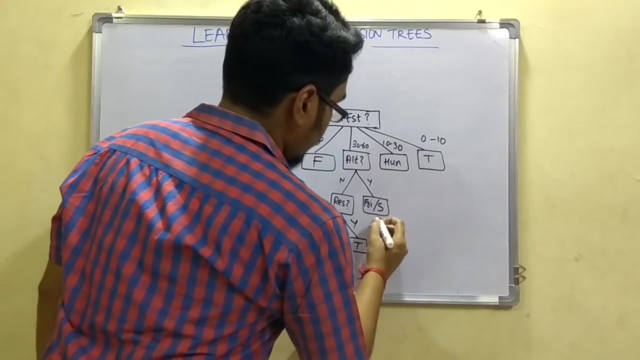 not satisfied and we would roll back and go to some other node and we will further explore this decision tree. and next is we have now this has ended here. so this left subtree has been ended. now we'll move on to the right subtree. that is, when the day of the week it is a Friday or a Saturday. so for that we have. 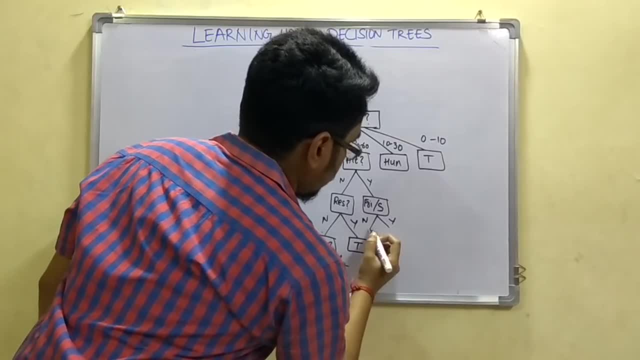 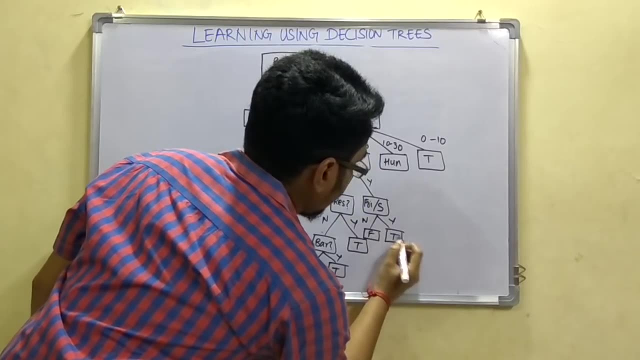 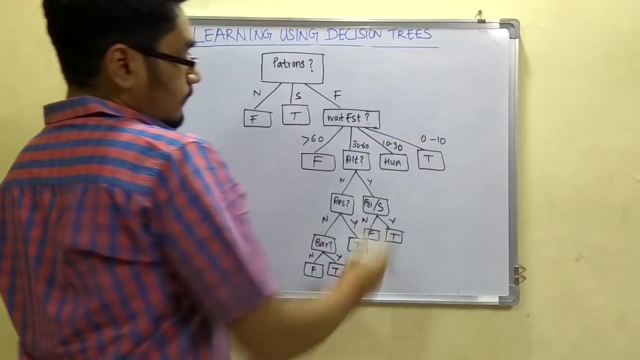 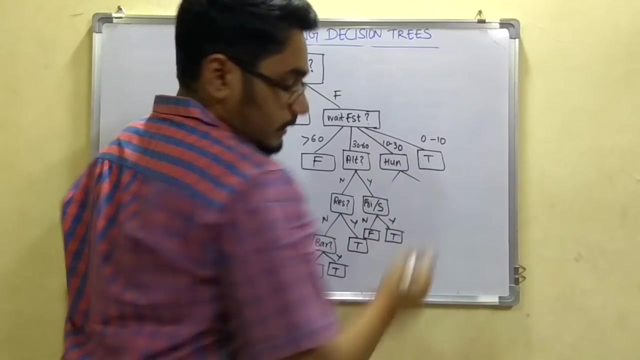 two, that is, whether it is yes or no. if it is no, then we have the F and T: for yes, it will always be true and for no, it will always be false. next, we have completed with this alternate tree. now we'll move on to the hungry node that 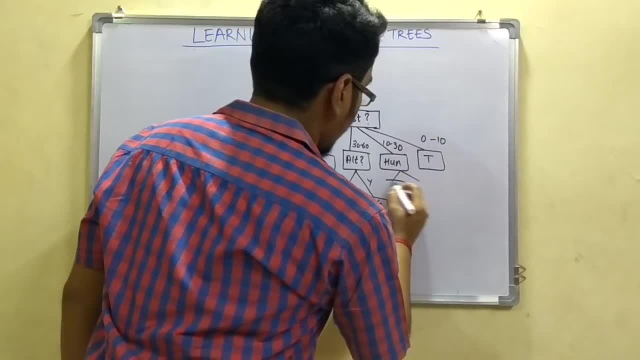 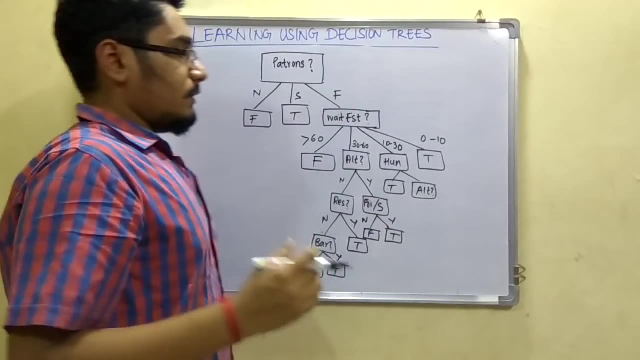 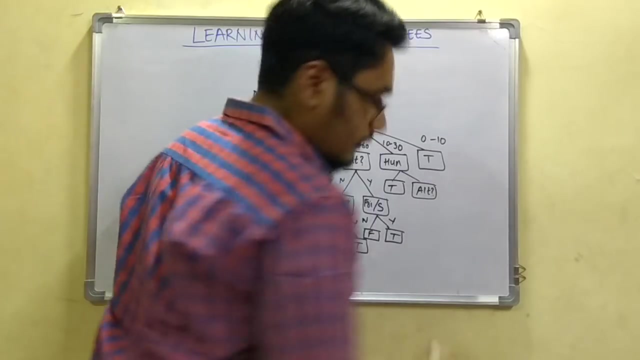 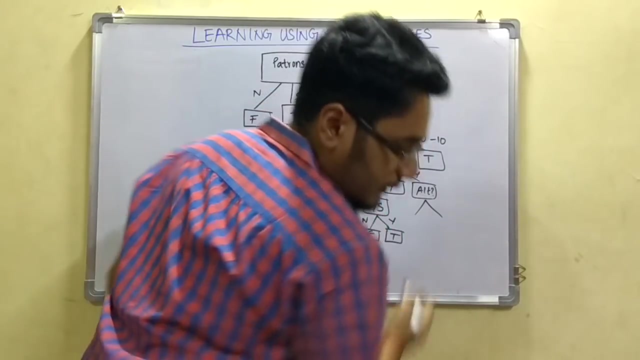 whether the patrons are hungry or not. so for that we have the T, T, ALT and ALT. that again, if they are hungry, then they will move on to some other restaurant or alternate restaurant nearby. so it is also under no or yes, and the alternate is being also divided into no and yes, and whether it is a T or 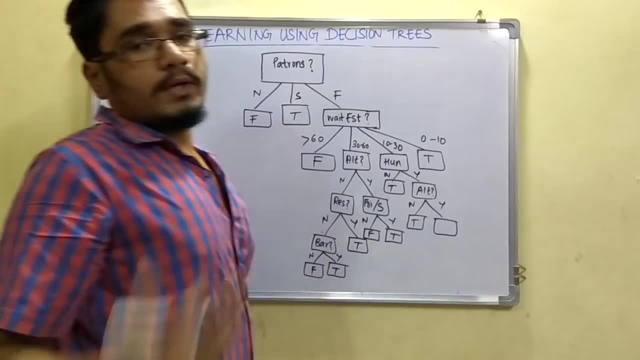 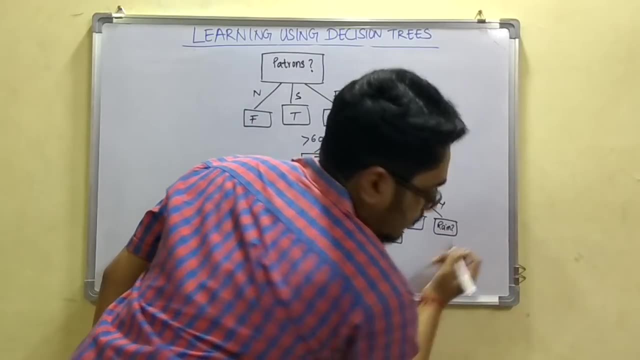 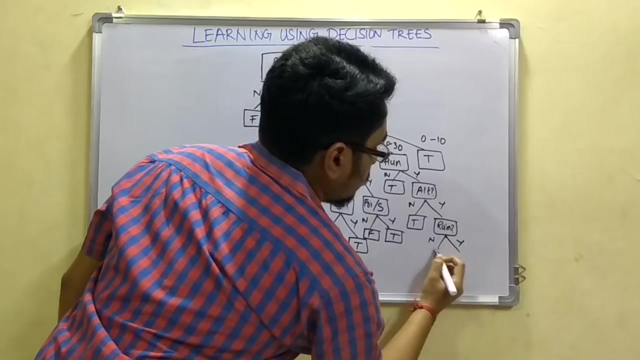 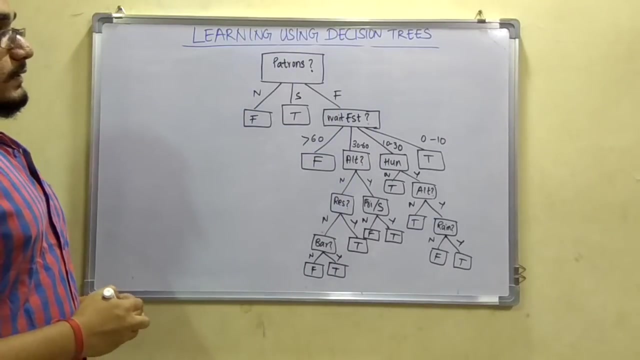 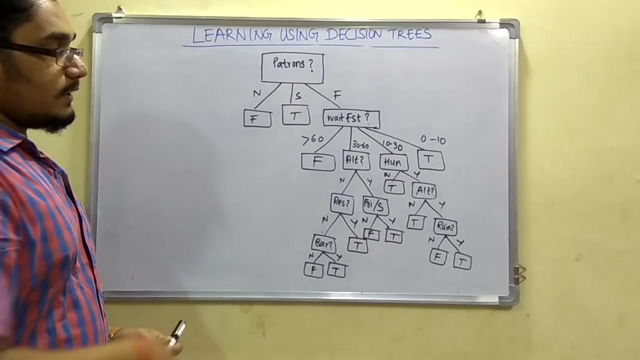 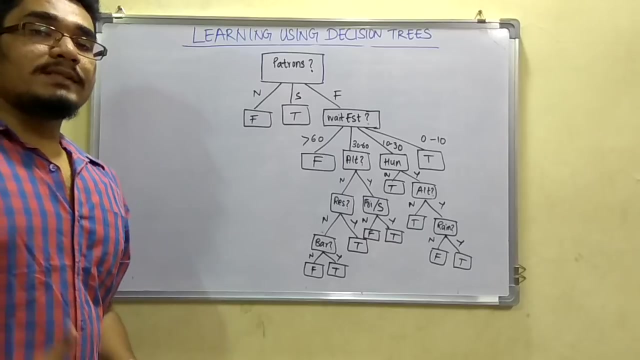 whether it is some other node. now other node can be considered as the ec. cool also, of course. you're getting free workloads sometimes. also an option may be. the robot can easily find out whether the goal state has been achieved or whether it has to wait for the estimation. so this is the overall